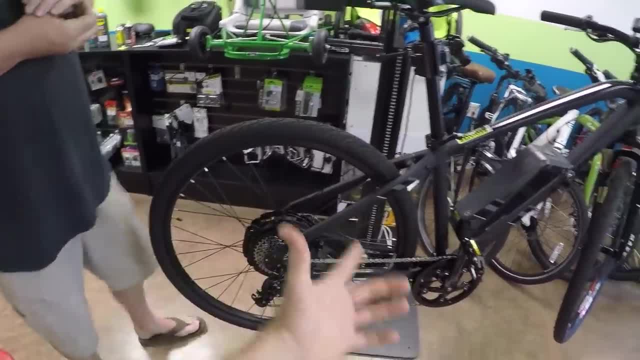 Okay, Good to know. Okay, So that's one of those again like a finer point, It depends on how you ride, your body type, all that. So I don't know. We want to start off with the drivetrain on this. 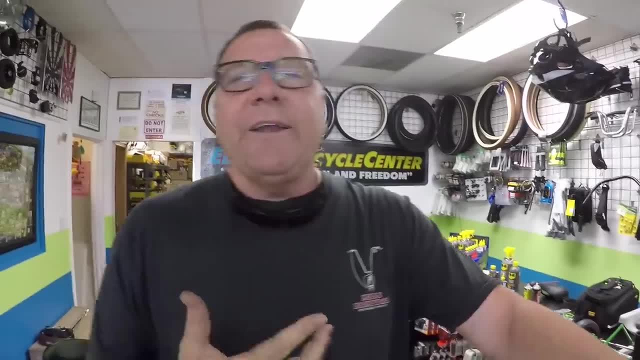 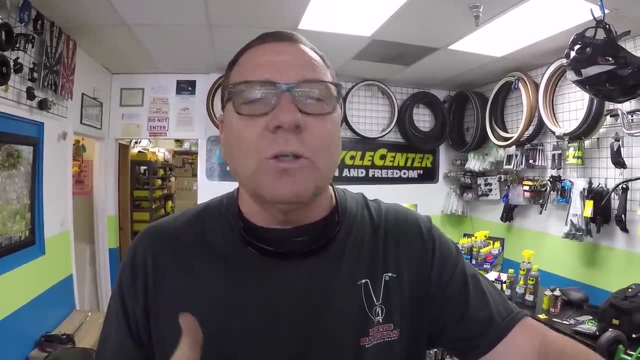 since that's something everyone that, Let's start with this. What can I do at home is what most people ask: Perfect. What's the maintenance that I should do? What's the maintenance that I should do? So there's two things I tell customers, Of course. keep your battery maintained. charge your. 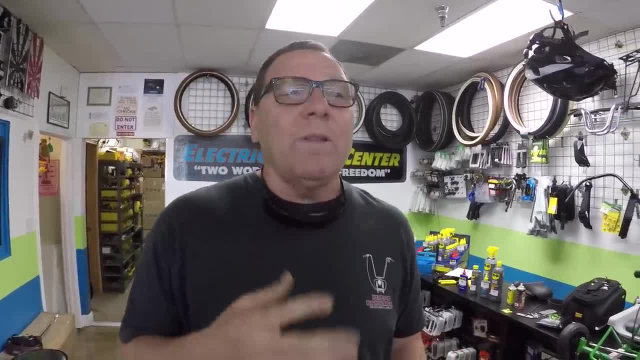 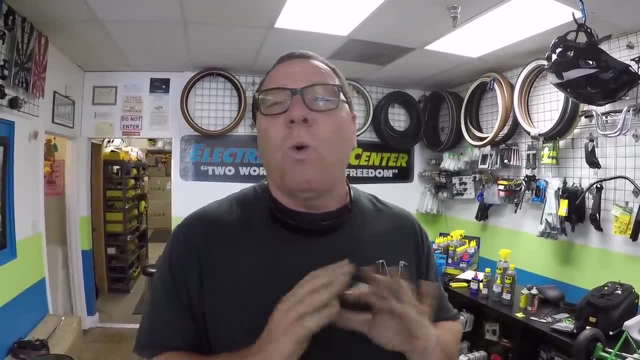 battery. Duh, that's a no-brainer. The second most important thing in my opinion on an electric bike- and I've literally had a lady drive an hour and a half to come to my store who swore up and down her battery was defective. it was bad. you can't even go 100 yards and my bike shuts down. 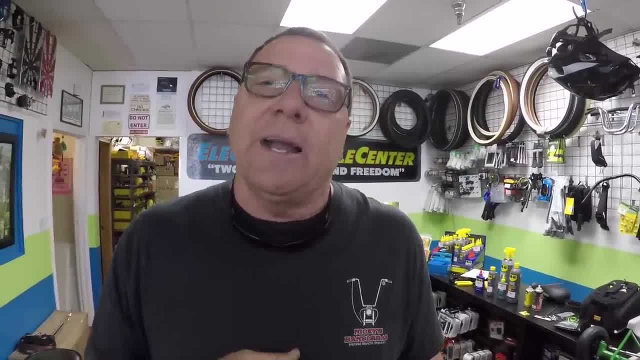 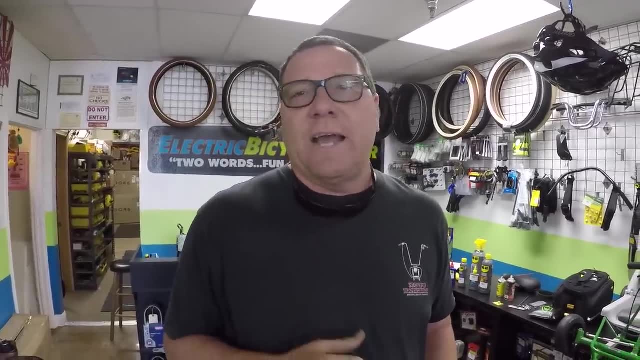 She showed up with her bike with 18 PSI in her tires. Oh, You've got to keep your tire pressure maintained, and bicycles lose tire pressure very quickly. I cannot stress that enough. That's true, And with changing temperature I think that can kind of deflate the tire over time. 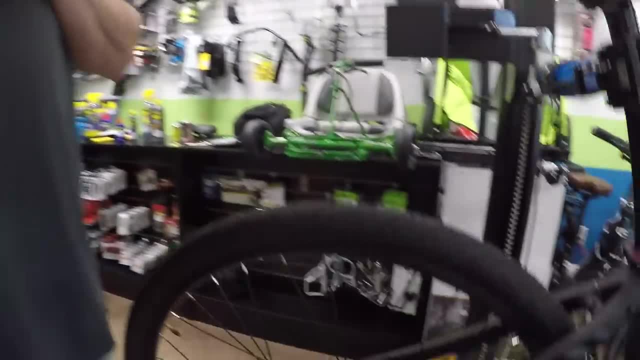 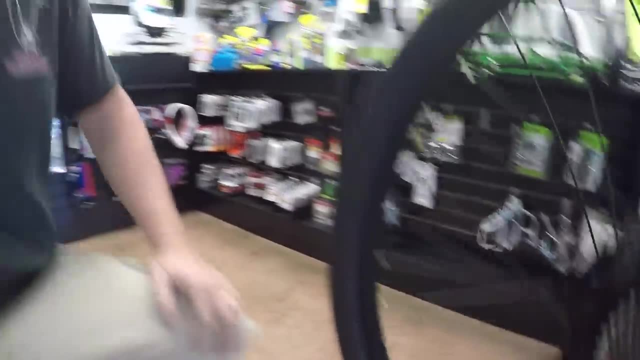 You say PSI pounds per square inch. Yes, So you know, make sure that you read in your manual, or even on the side of the tire, how much tire pressure you should have in there, And I would say every two weeks, maybe even three weeks. 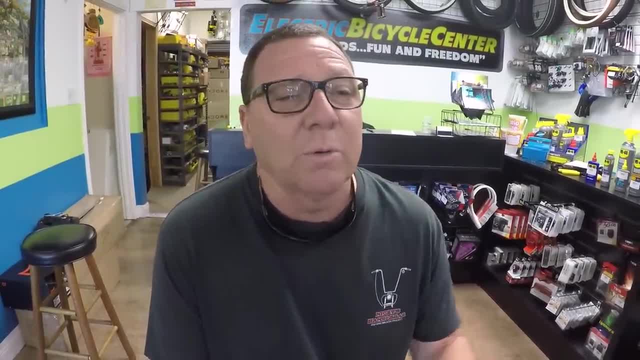 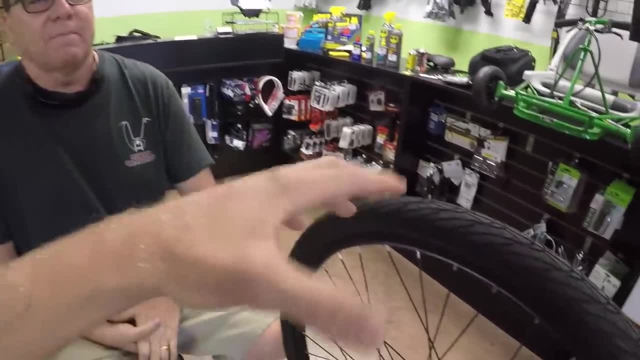 a minimum once a month. you got to check your pressure, or it'll start to affect the range, it'll start to affect the performance and the handling. everything else Can't even get a pinch flat Right Where, like you hit a curb or something and it kind of pops your tire. 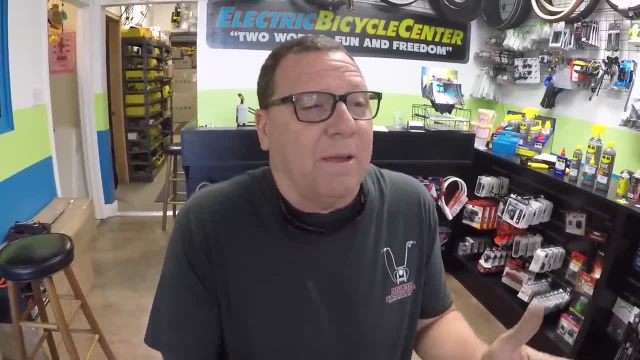 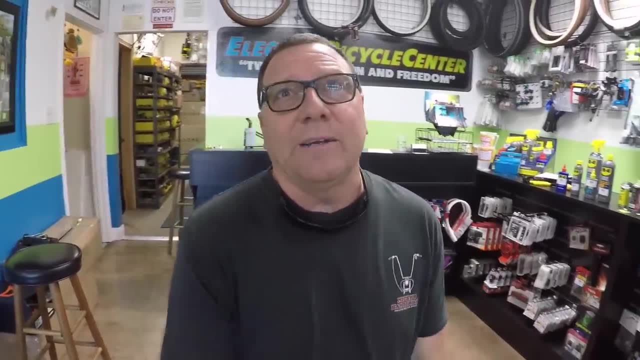 Absolutely, But even more so. I've literally had people come in and they're like: hey, my bike used to go 20 miles, now it's only going 12 miles. what's wrong It's you've got low pressure in your tires. 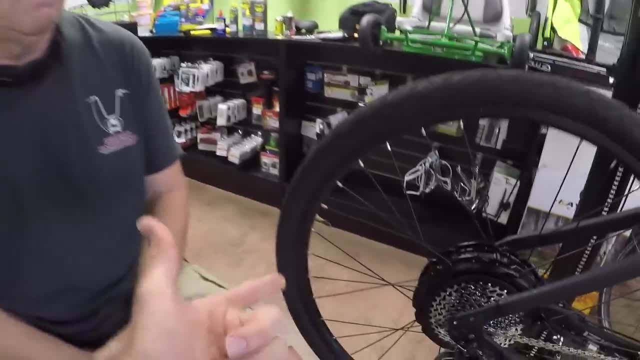 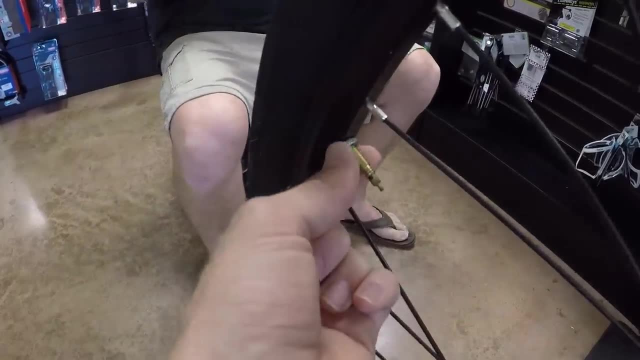 Okay, That's a good one. Thank you. Thank you, Absolutely. Maybe, while we're on that subject, did you have, like this is called, a Presta valve right here, right, So it's a little bit skinnier and it's usually got this sort of locking twist nut here. 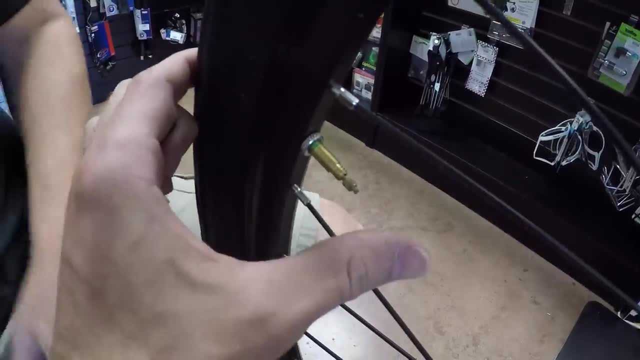 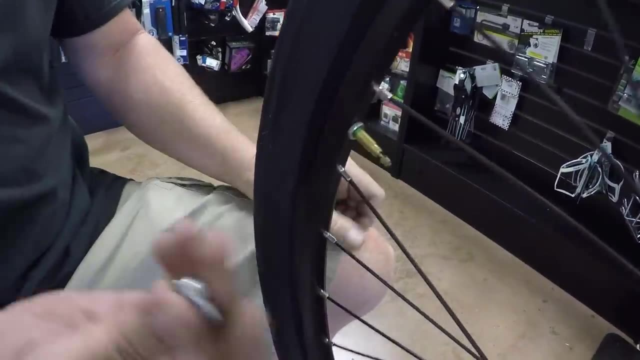 To inflate this, you actually have to unscrew it a little bit Like that, right, And you can even take that all the way out. Well, this one, you just back off and you can release air pressure And then to put air pressure in some of the hand pumps you can put directly on here. 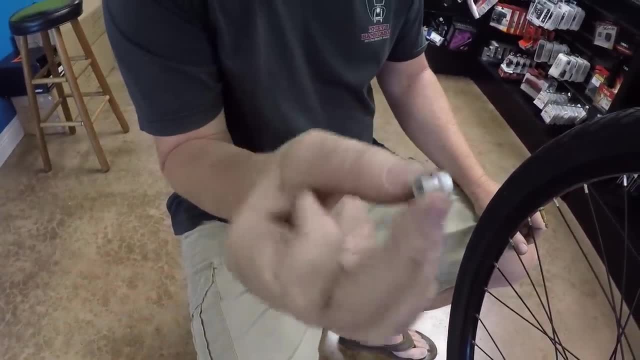 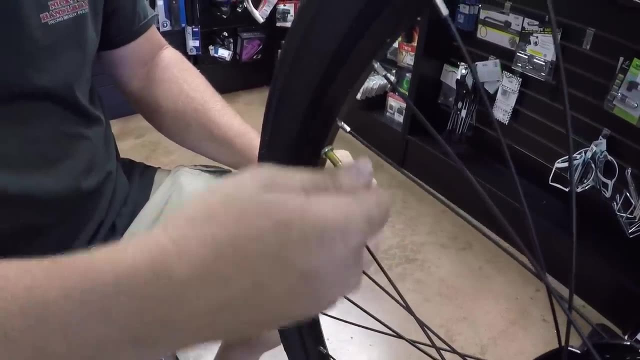 Or if you're more, conventional tire pump has a Schrader valve. you put this adapter on there, screw that on Now. make sure that you loosen this first. Yeah, If it's tightened down and you put this on there and you can't put air in there, you're calling me up going. 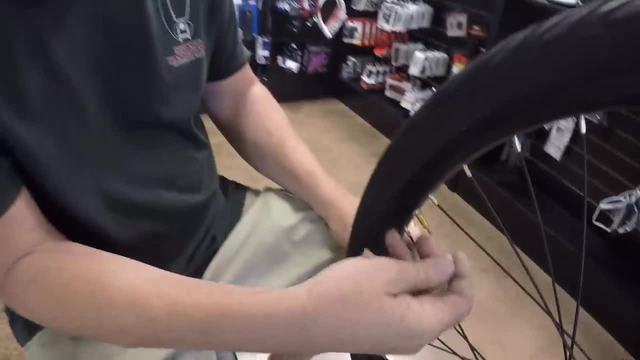 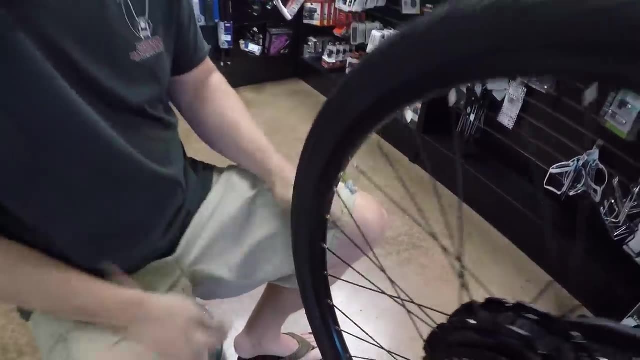 why can't I put air in my tire? You got to loosen that little bit. Yeah, You got to loosen that little cap up first and then put this on there and then tighten this down, and then you can pump it up. Okay, great, great. 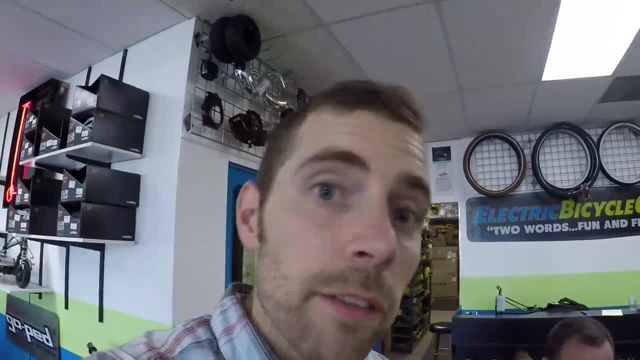 A lot of bicycle pumps these days have. they're sort of adaptable, So you can have a Schrader valve or a Presta valve work with it, but that's worth calling out. If you go to a gas station, though, that's not going to be the case. 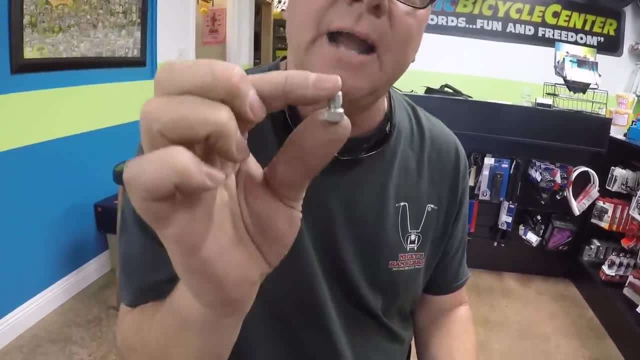 Oh, they only cause. that's for cars, right, And cars use Schrader valves. You need the little adapter. We give that for free to anybody that buys a bike that has that type of stem on it. That's nice. 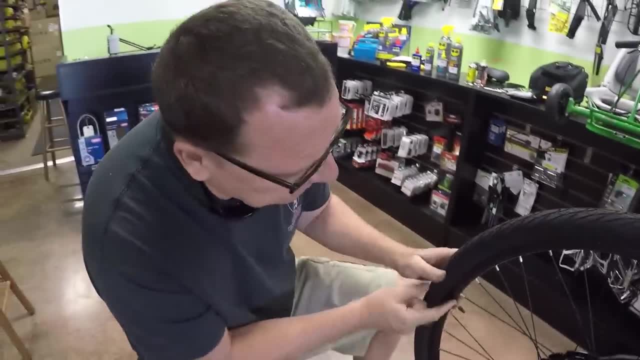 Make sure you put your cap back on there. Tighten down the cap all the way, Yeah, And also make sure that this is tight too right here, Yeah, Get that nice and tight against the rim as well, Okay, great. 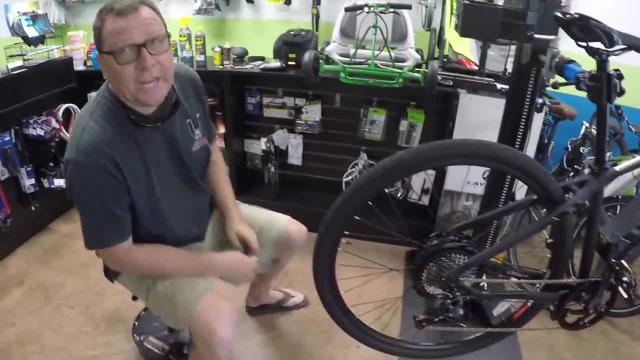 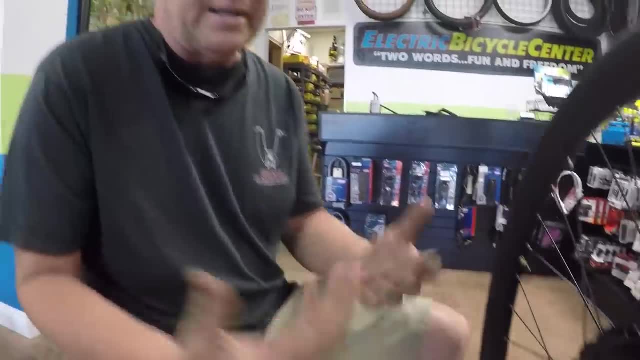 That's that Next probably would be your chain, And a lot of people can maintain their chain at home. You want to keep your chain clean and you want to keep your chain lubricated. I've had customers come in the shop and the bike still looks brand new six months later. 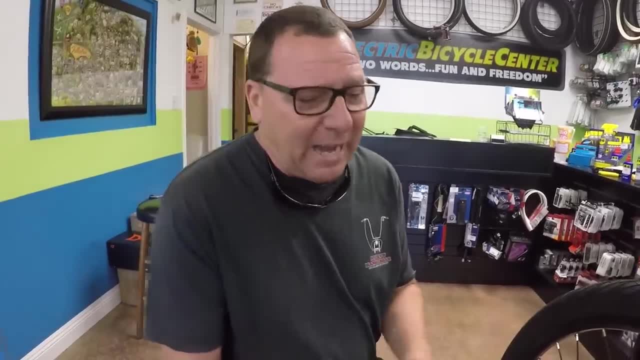 And I'm just totally impressed. you know, I'm like, wow, And that's an, A personality guy, that's really. you know, if you invest three grand in your bike, or even a thousand dollars in your bike, you want to maintain it. 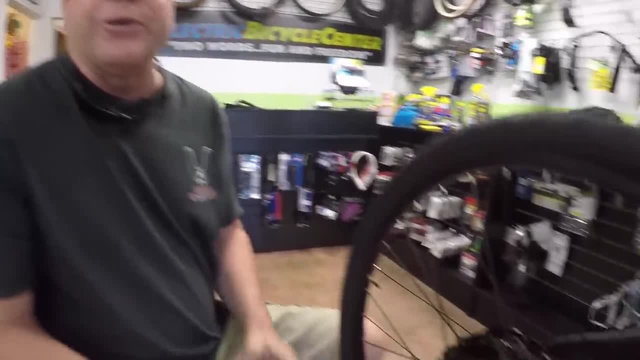 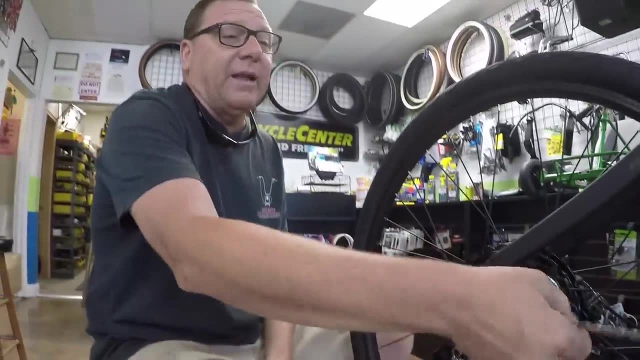 Some people don't do any maintenance whatsoever though. Yeah, They come in and they're dirty and you've got to clean the chain, and then you've got to lube the chain, And when lubing the chain, a lot of leftover lube will end up on the sprocket and in the derailleur back here as well. 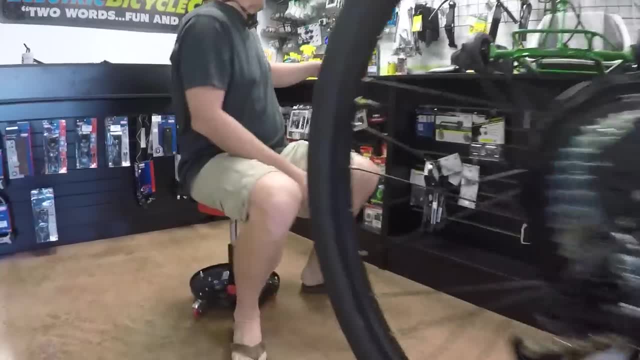 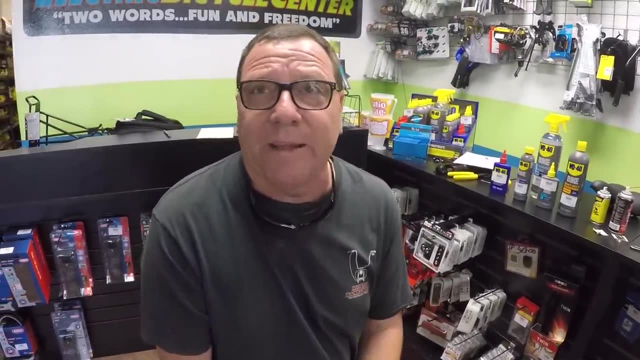 Okay. So what is lubricant? You know what are. So a lot of people are thinking: you know, I've got some WD-40 over here. If you use WD-40 in a spray aerosol, that is not a lubricant. 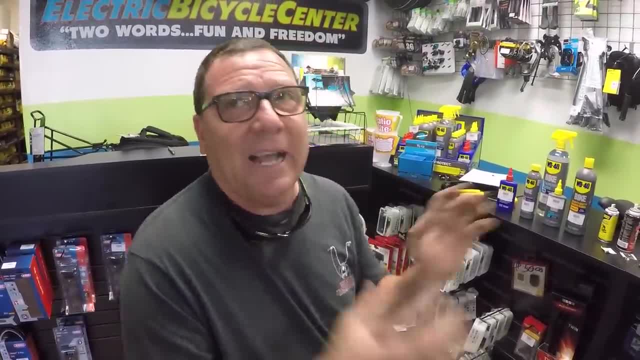 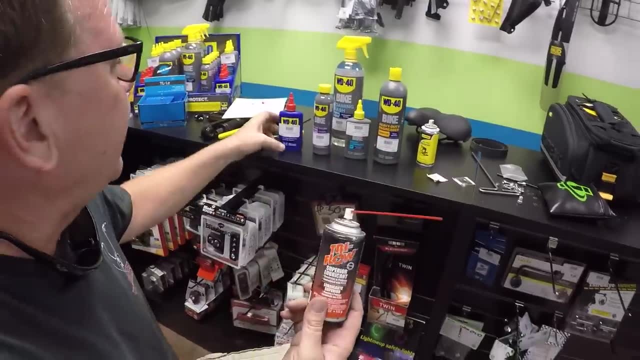 That'll actually dry your chain out. That's a penetrant, So don't get that confused. You have to use something that's a lubricant based. I sometimes will use Tri-Flow, and then WD-40 does make a product made specifically for lubing the chain. 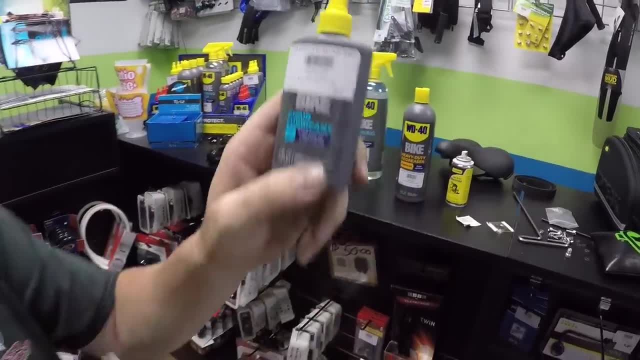 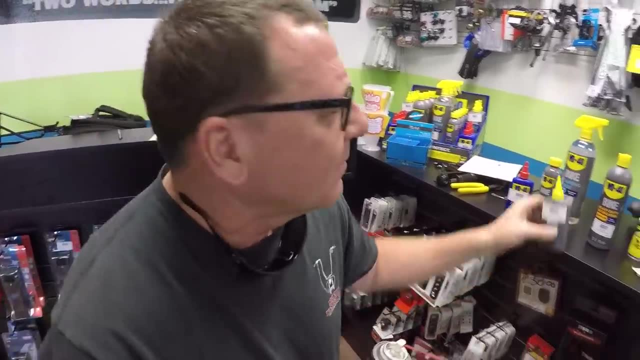 There it is And look for it saying chain lubricant, not penetrant. You can use a penetrating oil to clean the chain and then follow that up with a lubricant. Okay, Excellent, That's it. Another common problem on disc brakes is they squeak. 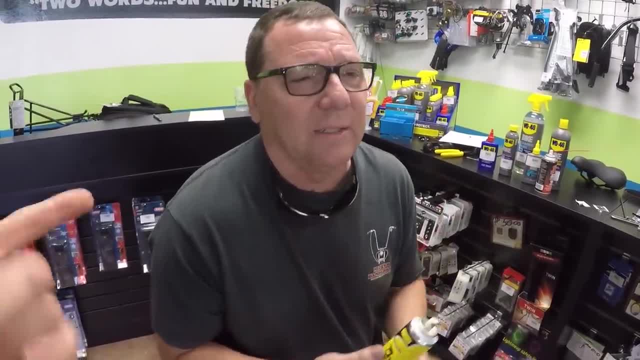 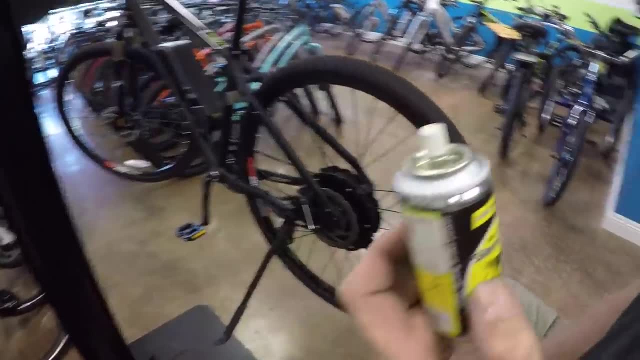 Oh my gosh, it's driving me nuts. My brakes are squeaking like crazy. People say that Yeah, I hear that a lot. Take your caliper off, take the pads out, spray them down with a disc brake silencer. 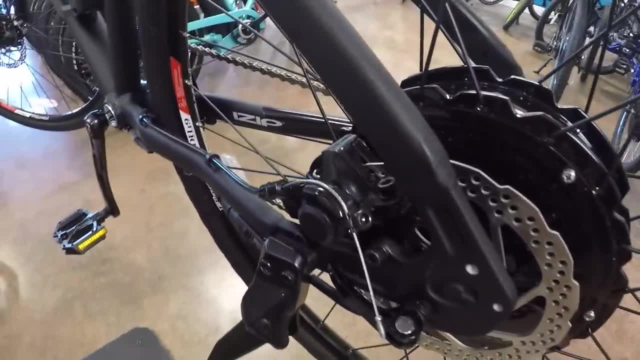 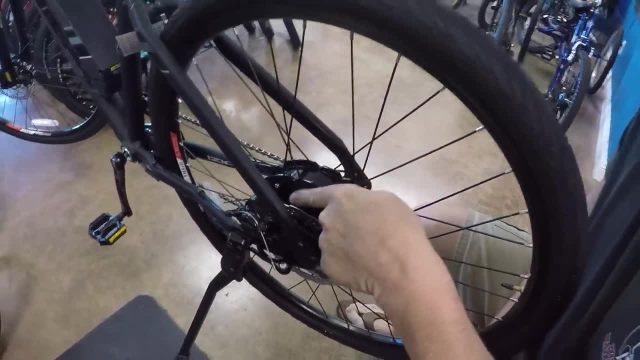 something that'll keep them from squeaking and that sometimes will do it Nine times out of 10, though it's just an adjustment And to adjust the brake you can actually do a visual down it, And a lot of times there is adjustment on each brake pad from the backside or the front side. 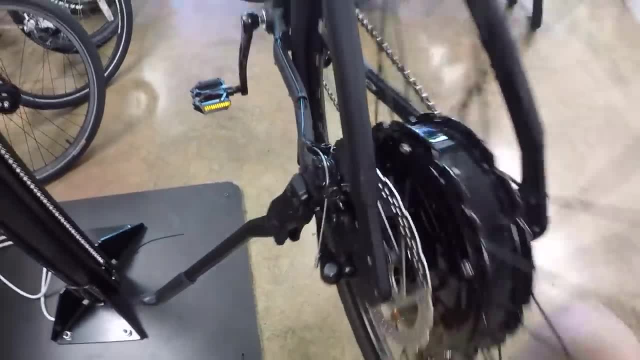 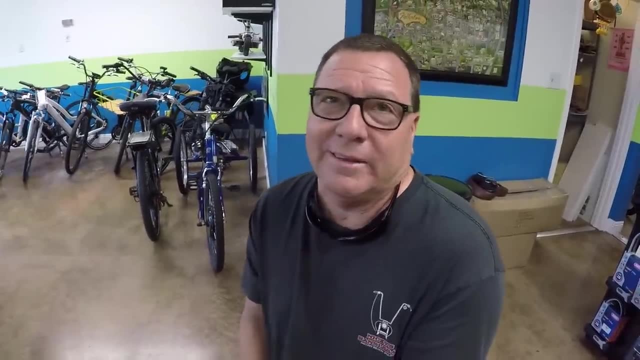 And you want to align that so that the wheel spins freely and it's not dragging. That's awesome. I definitely heard it before- where it's like ka-ching, Ka-ching, ka-ching And if you have a slightly bent disc it's difficult because once you get the squeak out, 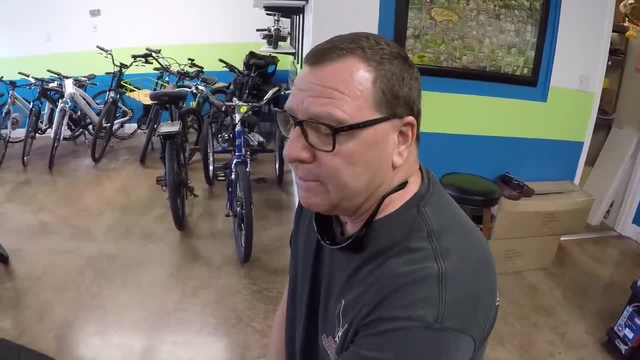 then the brake's adjusted so loosely you're not going to stop At that point. it's time to either straighten the disc or replace the rotor, is what they call them. Okay, You got the rotors, you got the brake pads. 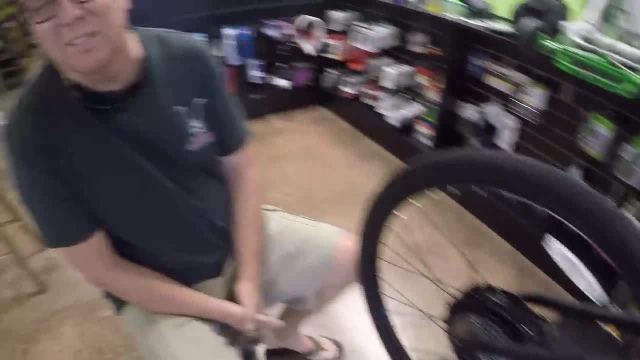 Eventually, are they meant to squeak to let you know like, hey, you need new brake pads, like in cars? Not really, no, I mean if you get it all the way down to the point where it's metal on metal, but I rarely ever see that. 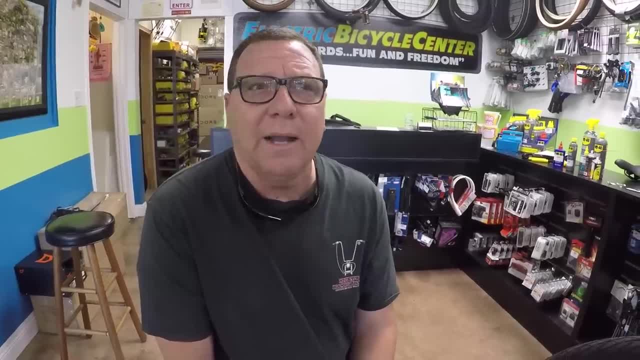 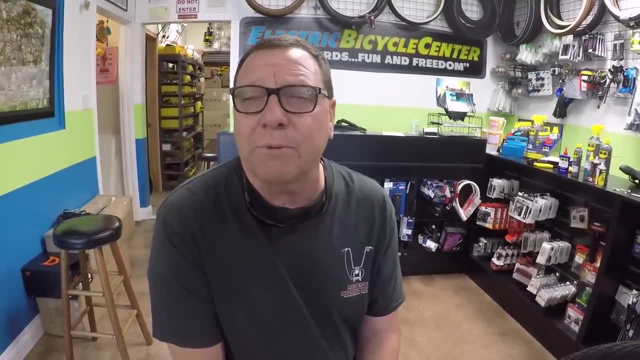 Most people are going to come in and we're going to point it out to them before it's to that point. Okay, And the brake pads last pretty long on bicycles. I have bikes that have gone 4,000 miles and they're still on the same original brake pads that came from the manufacturer. 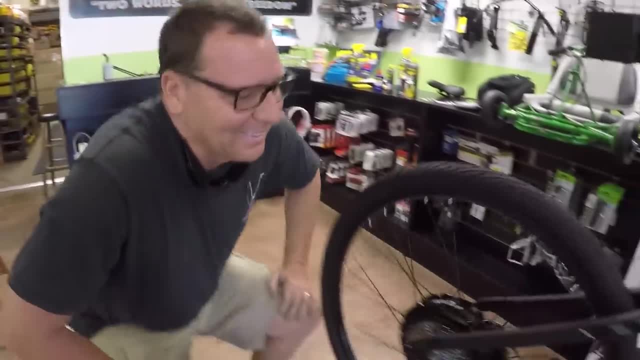 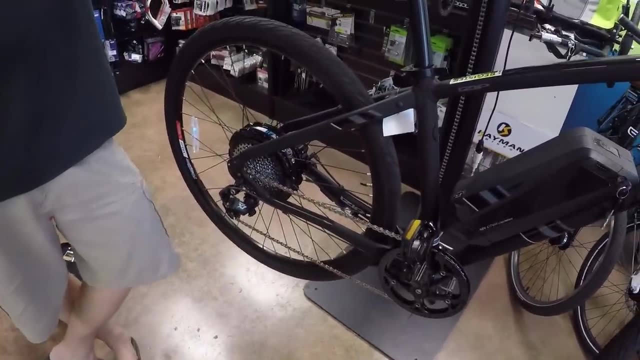 We call those guys adrenaline junkies. No brakes, they're just flooring it the whole way. Sam, while we were talking about the chain earlier, I wanted to reiterate that, yeah, you know you use the proper lubricant, but you're not supposed to have this thing be like wet to the touch, right. 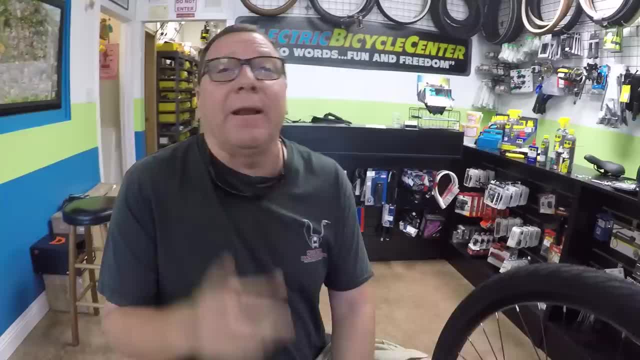 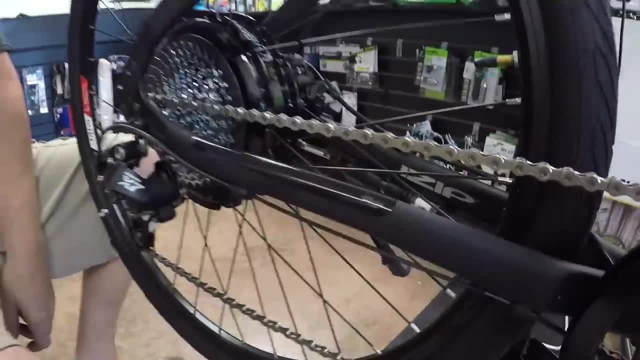 You like want to wipe that off afterwards? Yeah, but on the other end of that, the other end of the spectrum with what you just mentioned, Cork, I have people come in. if I can grab your chain and my hand doesn't come back with some kind of lube on it, it's totally dry to the touch. bad news. 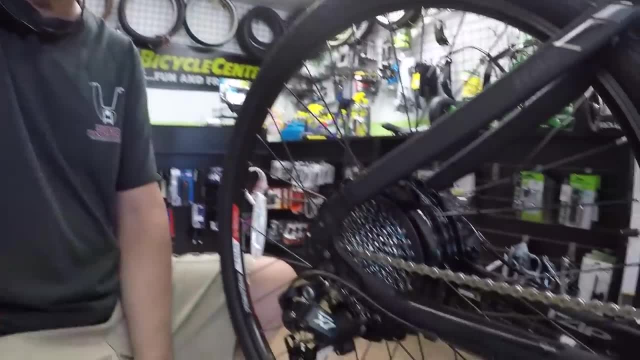 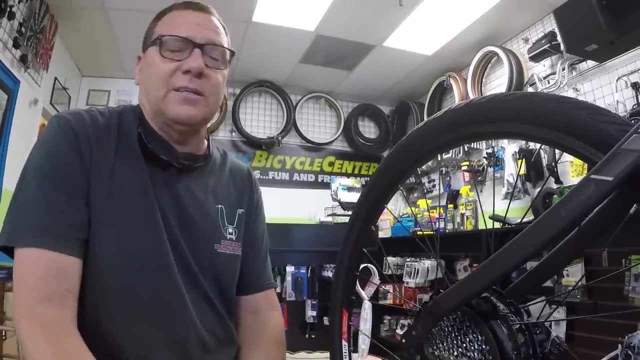 You've got it way too dried out and it's time to put some lubricant on it. So there's. you can have it too dry or you can have it too wet. I like to actually see a chain a little bit on the wetter side than the drier side, because it's keeping it all lubricated. 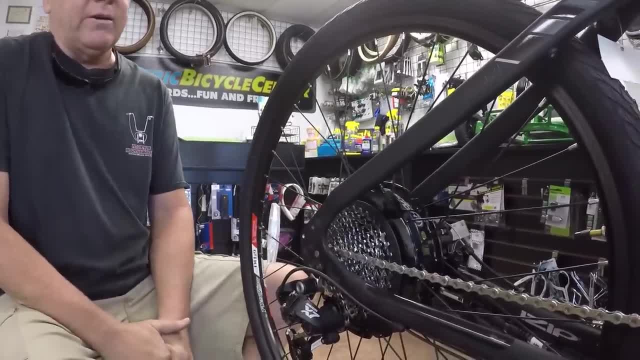 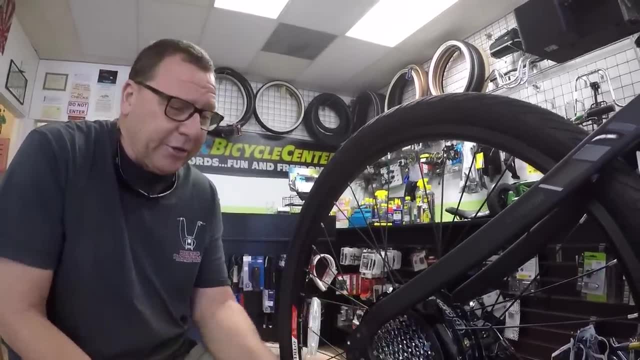 But what does that do? Like, it just keeps it from rusting. or you know, Not only does it keep it from rusting, but it gets a little bit of cushion between metal on metal. I mean, this is a metal chain, a metal sprocket. 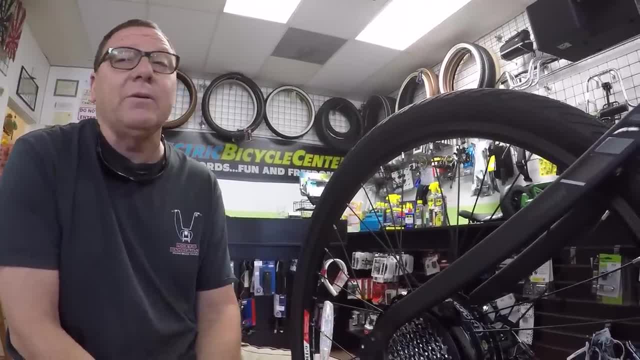 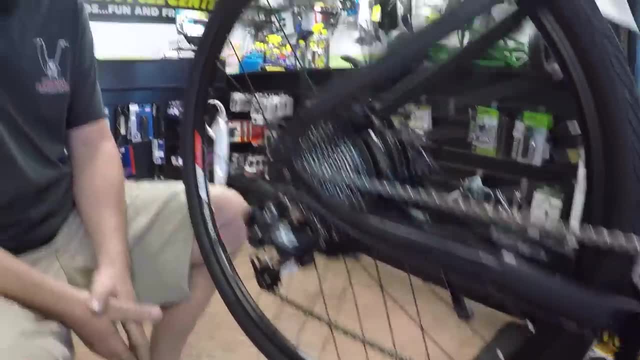 You're going through your derailleur down here. You want to keep it. you want to keep it lubricated. definitely, Okay, that's good to know. Any other tips on the drivetrain, Like what happens when someone starts to hear like kind of a crunching and it's not shifting? 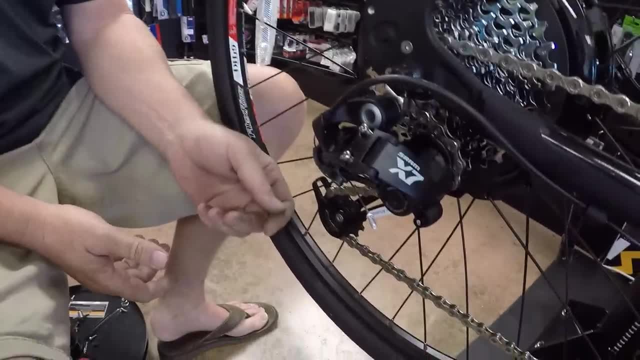 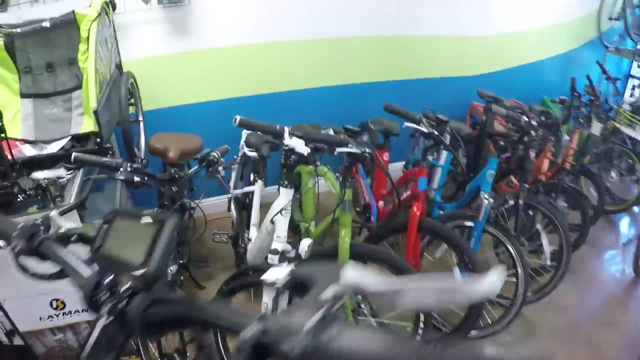 Your derailleur is just slightly off and nine times out of ten it's just an adjustment on the cable that you can do. In this case there's no adjuster here. It would be probably up on the handlebar, So that's like up here where the kind of the shifters are. 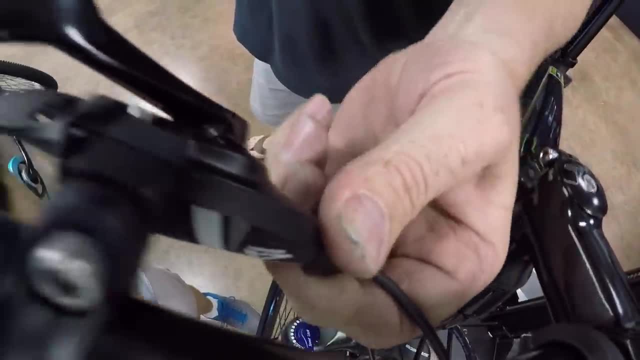 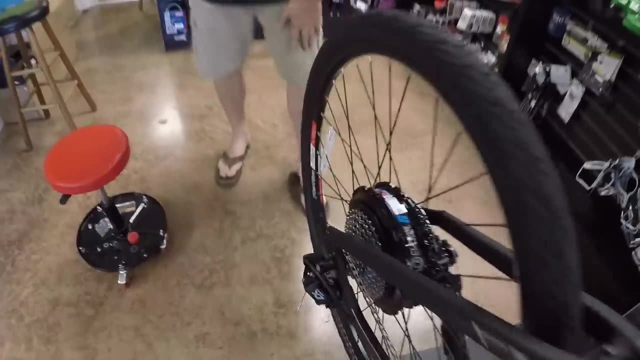 Yeah and see that big knob right there. You can sometimes just turn it one direction or the other direction to get rid of that crunching sound And you're just lining up the derailleur back there. You can actually do a visual If you come back here and you look directly behind the bike. 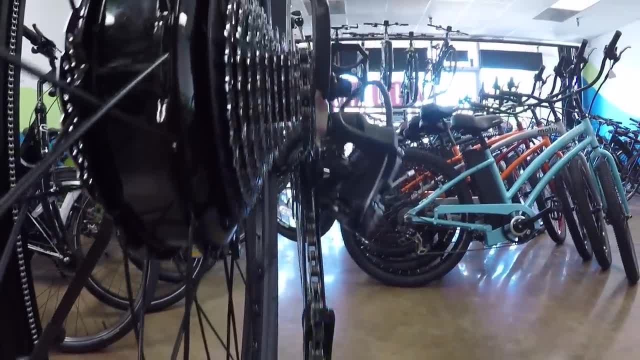 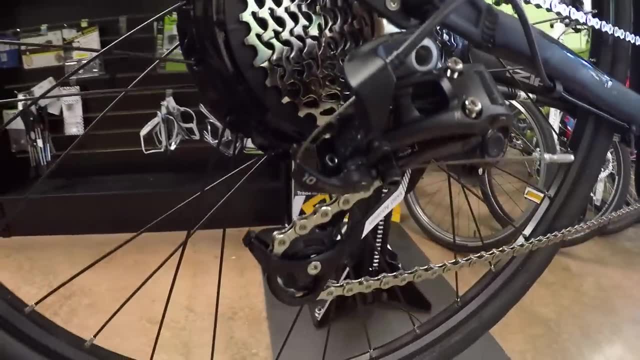 if you look at the chain and you look at the gear, it should be pretty well lined up And if it's pulling a little to the left or the right you just have to make that adjustment to line it up. Another thing you'll see sometimes is somebody will load their bike in a car. 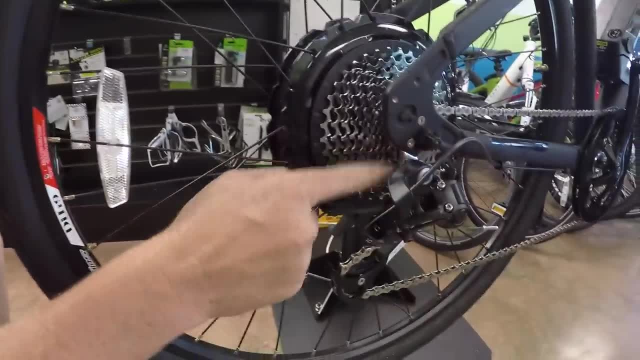 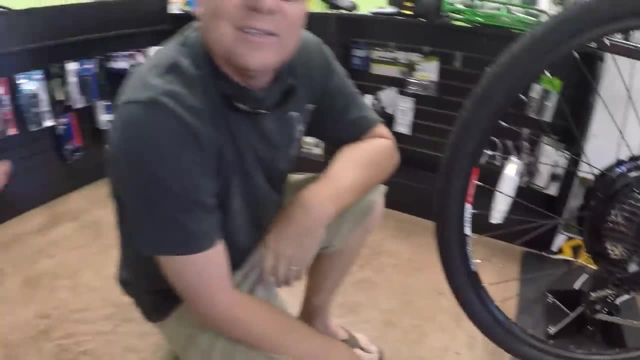 or they'll drop their bike and they'll bend the derailleur or the hanger here, And that needs to be straightened out, And sometimes I literally just grab it with my hand and get it a little bit straightened out. Pretty big guy, though. 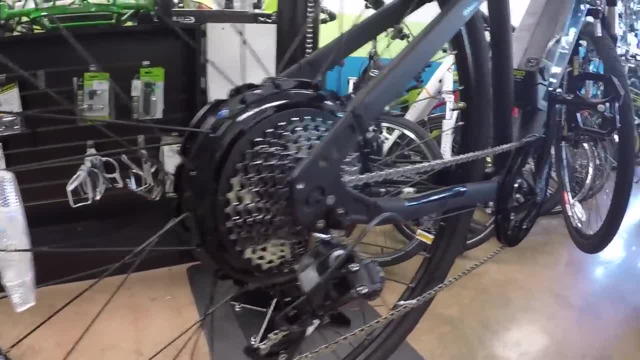 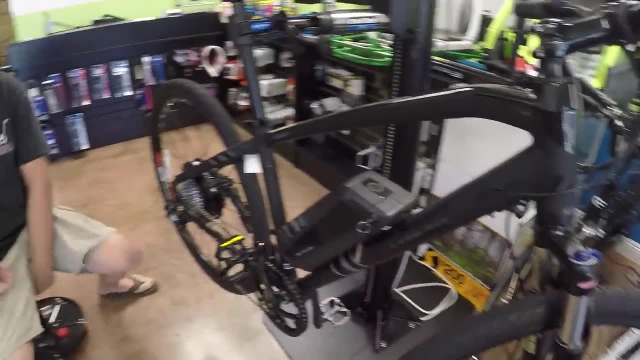 As crazy as that sounds, That's awesome. It's just getting it lined up, you know. Okay, Okay, great Common sense there. Let's move forward onto the bike. I want to show you something else, especially when you're prepping your bike and you're getting it out of the box. 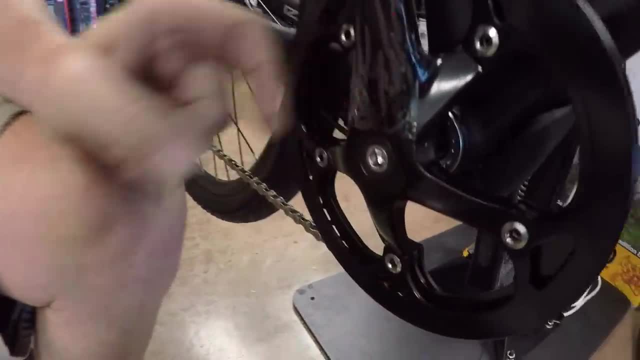 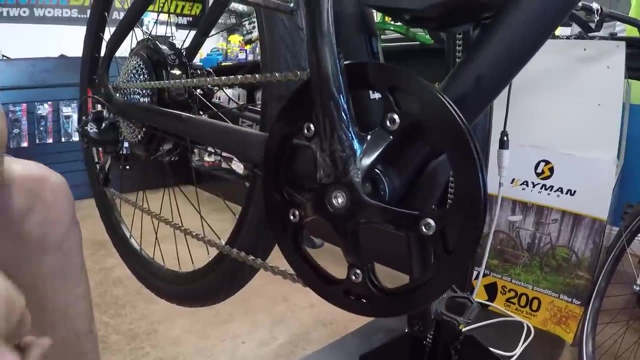 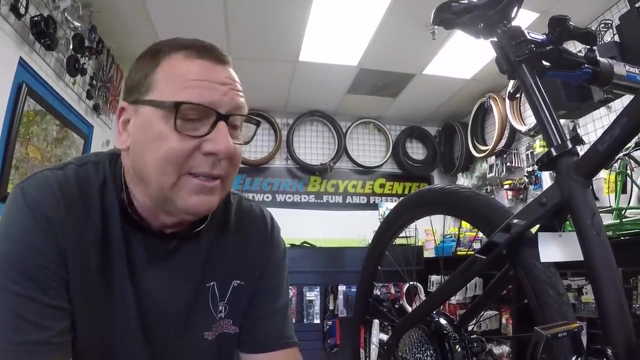 On certain manufacturers, your bottom bracket and your crankset. these bolts are not tight And you've got to check those with an Allen wrench and make sure they're tightened up on there. On a yearly basis, we have somewhere between 15 to 20 bikes. 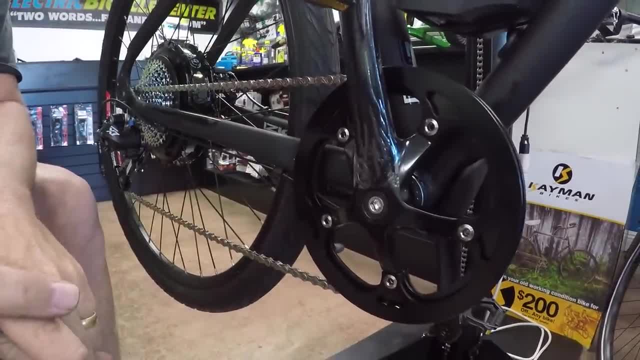 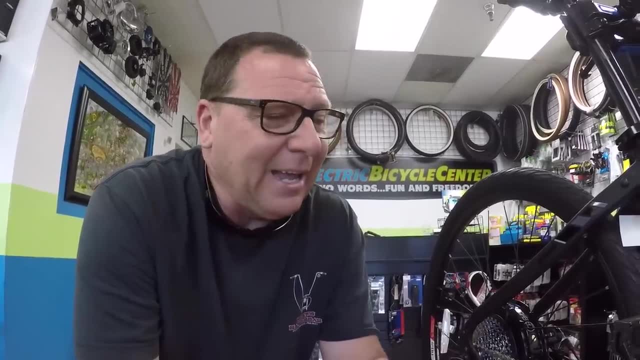 that an actual customer will take a brand new bike and the whole pedal crank will fall off on them. And I'm like, wait a minute. You know, on this particular brand of bike we've got to start double checking this stuff And we've gotten that number much lower now by prepping the bike and checking to make sure those are tight. 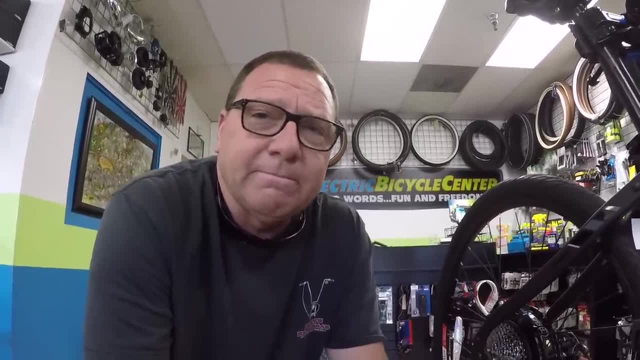 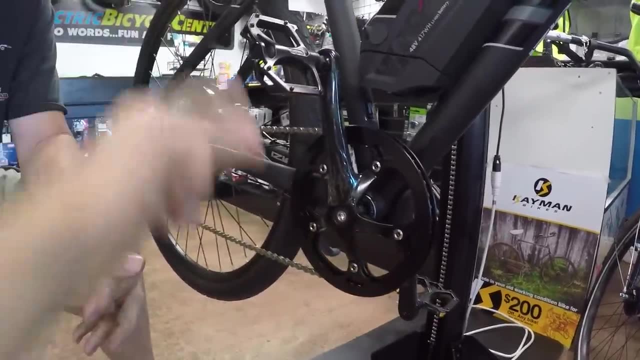 And you, as the owner of the bike, should be checking that as well once in a while. Thanks for that heads up. I've heard something about certain models, some with bottom bracket motors, like mid drives, and others with the hub motors, where things weren't tight and it kind of spun and rips the power cable. 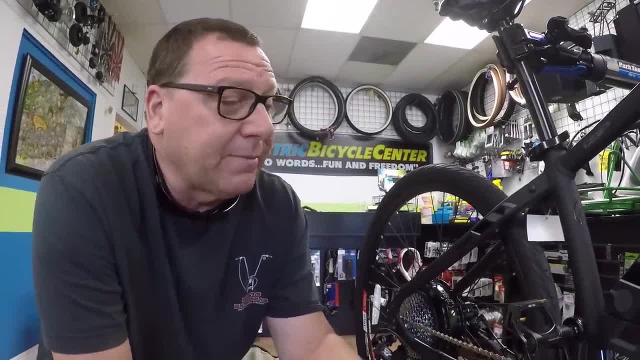 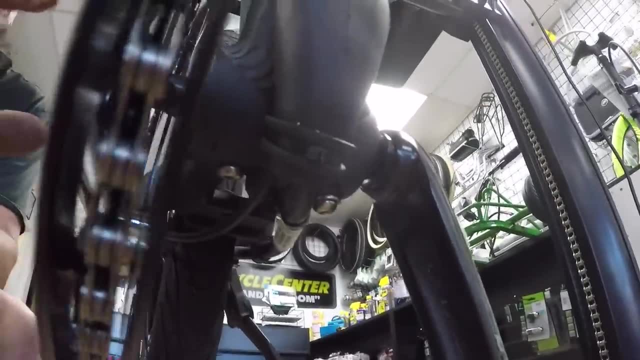 Have you heard? Do you know what I'm talking about? Yeah, actually, on the bottom bracket on this particular bike as well has a cadence sensitive sensor, I believe, And the wire comes in right from the bottom down there And if that bottom bracket's not tight it'll twist and that can cause damage. 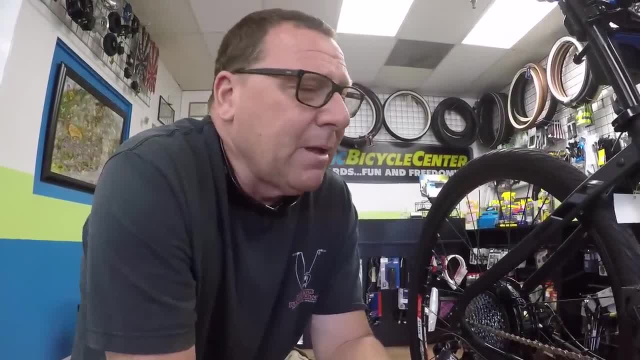 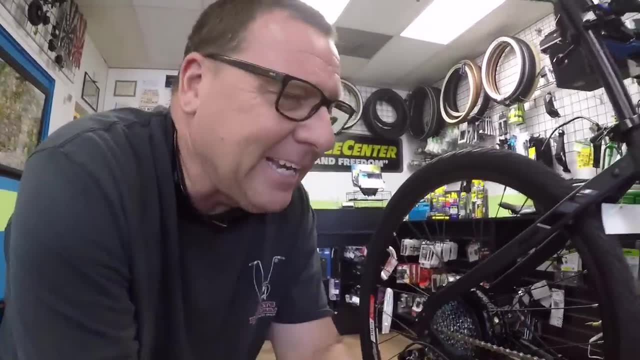 And then we have to replace that and get it taken care of. Other things that happen is: once a crank arm comes loose, especially on the bottom bracket, on a square taper, it ruins it And people try to tighten it. and tighten it ain't going to work. 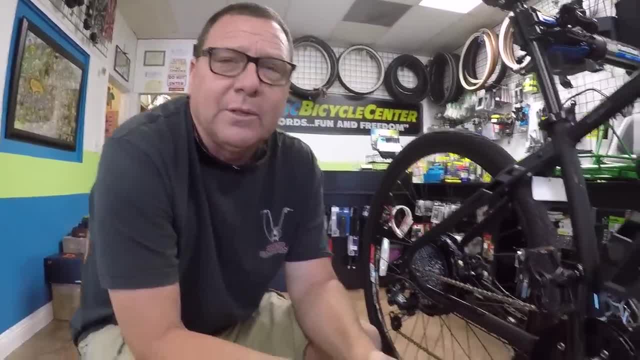 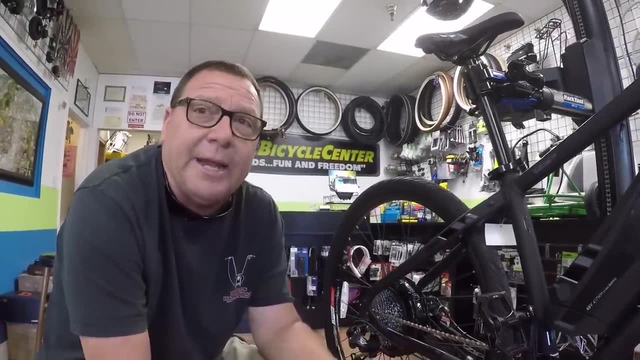 It's time to replace the bottom bracket and the crank set both, Which isn't difficult to do if you have the proper tools, And any bike shop should be able to do that. Not even you don't have to take it to an electric bike shop. 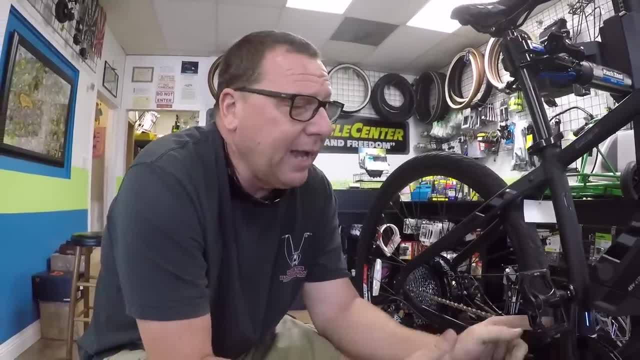 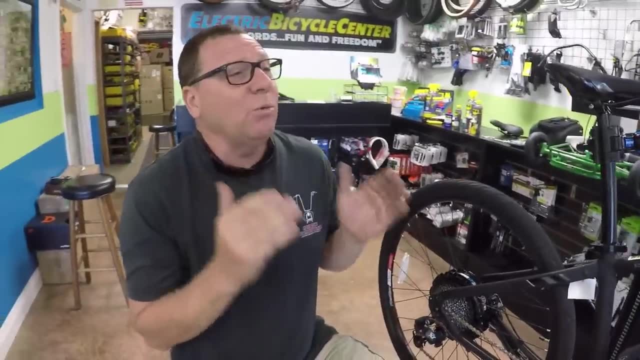 Any bike shop should be able to replace a bottom bracket and the crank set. Okay, that's good. Okay, now. another thing a lot of people ask me when they come into the shop is my Bob, is it waterproof? Can I get my bike wet? 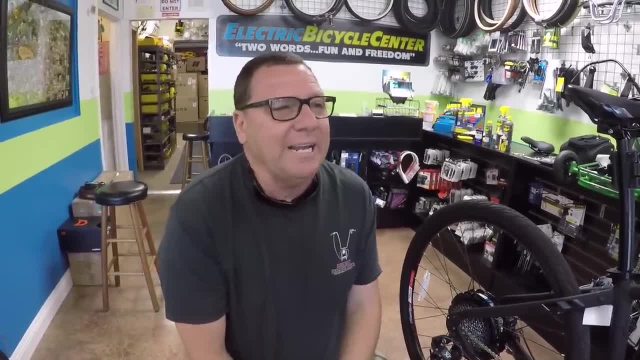 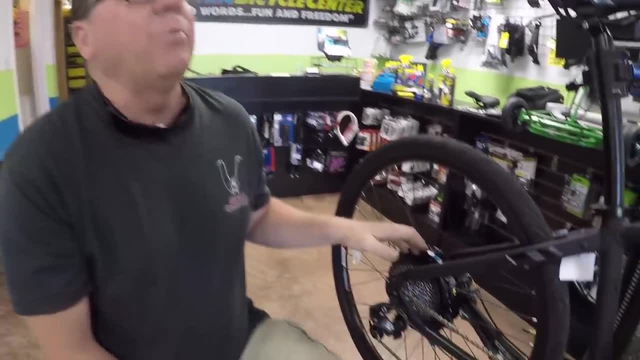 I'm afraid to even go through a puddle. You know what I would say? 95% of all electric bikes today that are on the market are water resistant, but they're not waterproof. The motor, no problem. Your display, your throttle, no problem. 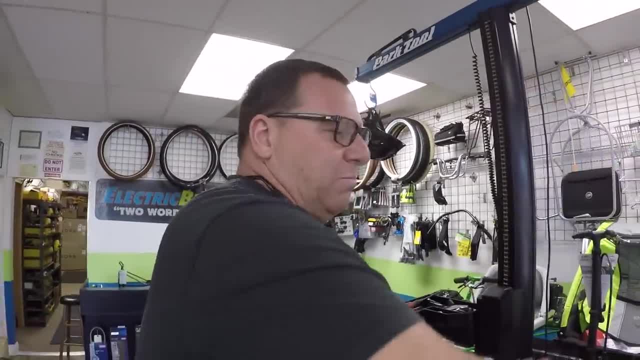 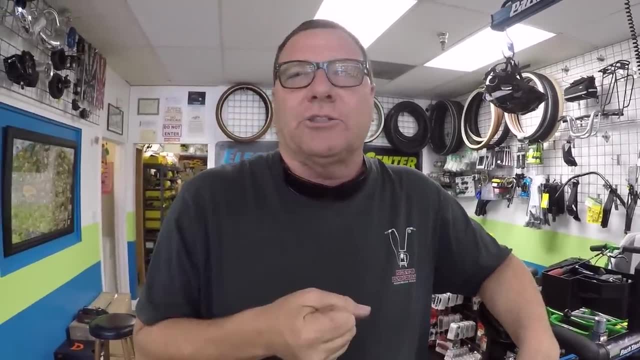 You can put direct water on it. I wash the bikes down with a sponge. I'm wiping this all down. In order for you to ruin an electric bike, you would have to take a pressure washer and hold it. I'd say the most vulnerable part on an electric bike would be the controller. 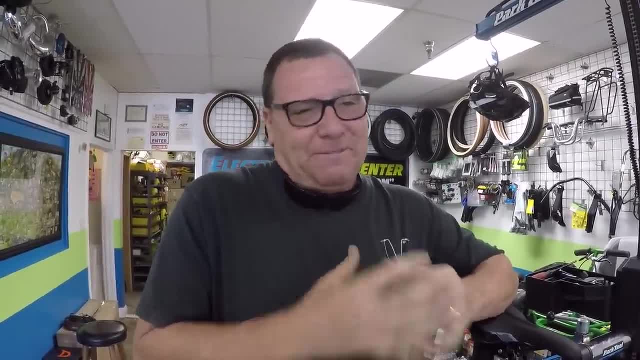 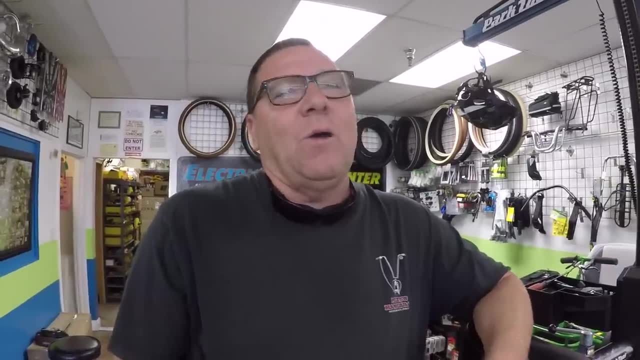 Right, Yeah, In order to get the controller to fail, you'd have to submerge it in water, So it'd be like your bike accidentally falls into the swimming pool. uh-oh, bad news: that could possibly kill it, And don't turn it on, right. 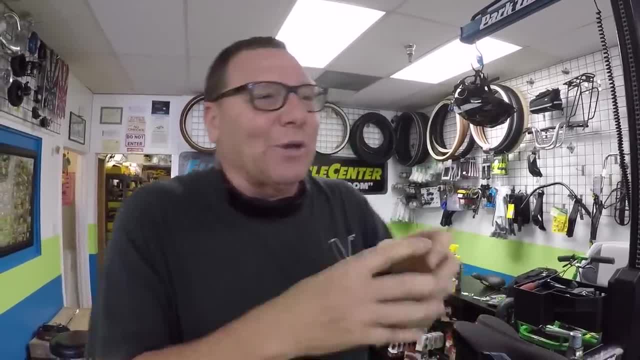 It's like your phone, like let it dry off. if something like that happens, Yeah, throw your controller in a bag of rice, right, Right, right. That's what I'm, and just so. this one, the controller, is so integrated you can't even 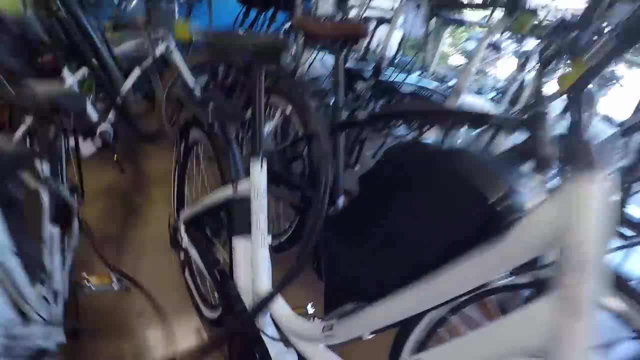 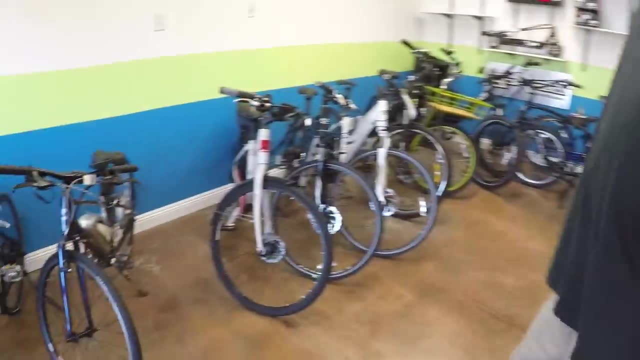 see it, but we had another e-bike over here. You can see this little control box back here. Here's the battery. There's the controller box. I don't know if there are any others that- Oh, there's lots of them that I can show you. 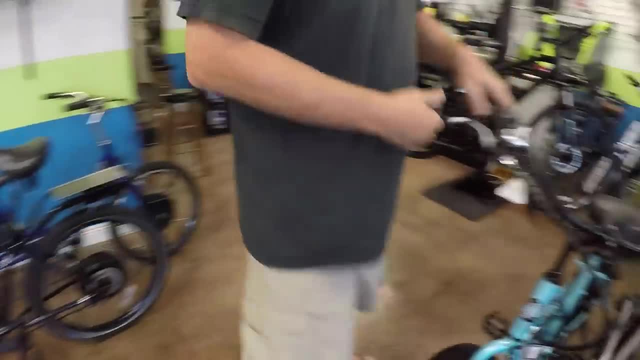 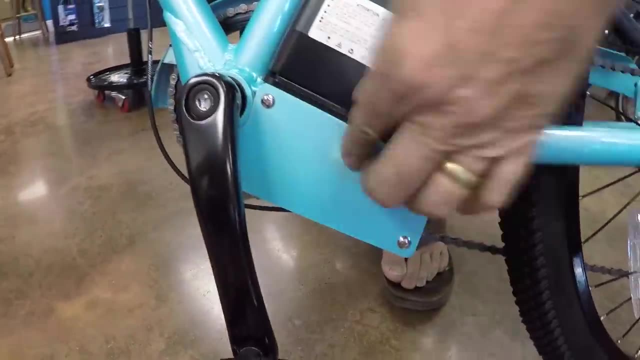 They're always in different places. Yeah, here's like on a Motiv. here it's underneath. this is a very common place that a controller is is batteries here. all the wiring for the bike comes into this box down here where the controller is located. 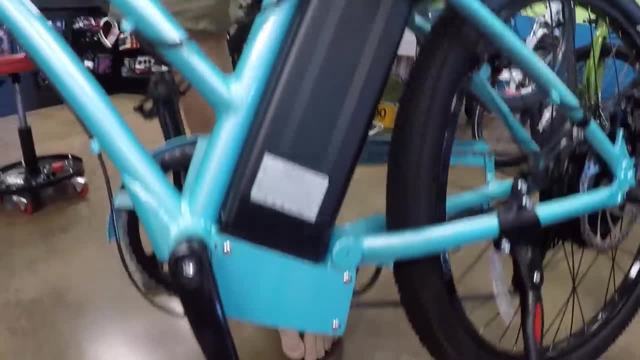 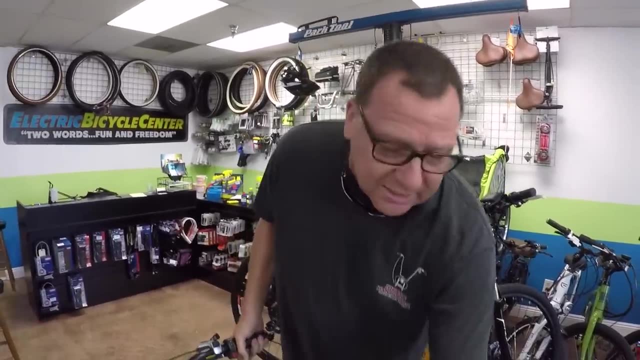 And you're like, oh my gosh, that's the lowest point of the bike. I've had customers ride these Motiv bikes on rainy days and literally have that practically submerged and it doesn't fill that box up with water. You might have a little bit of water in the box. 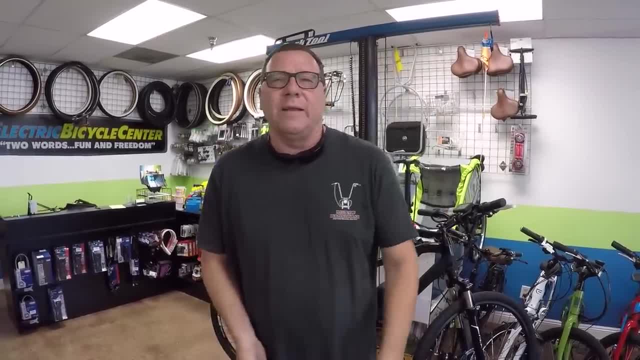 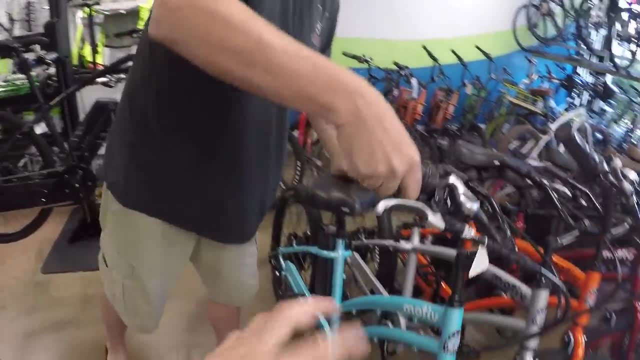 You might have water in the bottom area there and it'll dry out. Not enough to ruin the bike, not enough to kill the controller, by any means. Yeah, I've had some really nice road bikes and I was always just pretty careful about when I cleaned it. I used something like that WD-40 stuff. 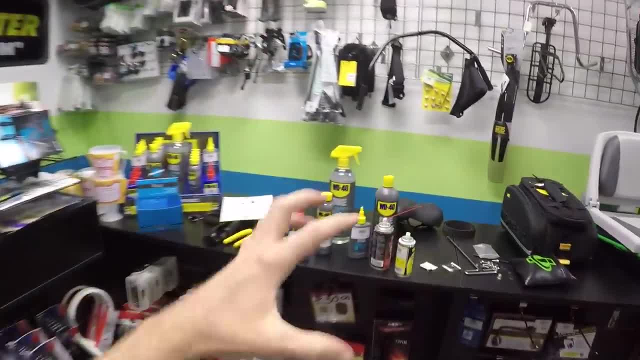 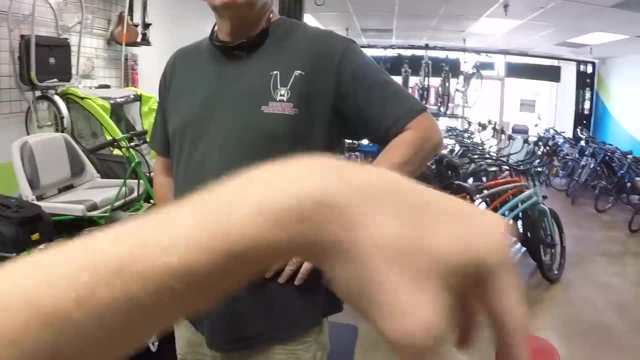 And they have eco-friendly cleaners you can spray on. You use a paper towel. I tended not to use my sprayer because people said, oh, sometimes water can get into your head tube or different places and kind of rust it or you know. 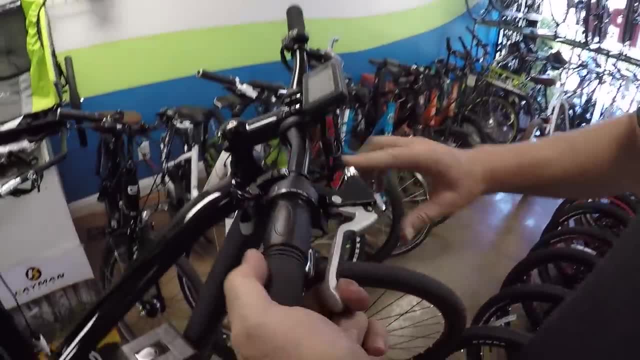 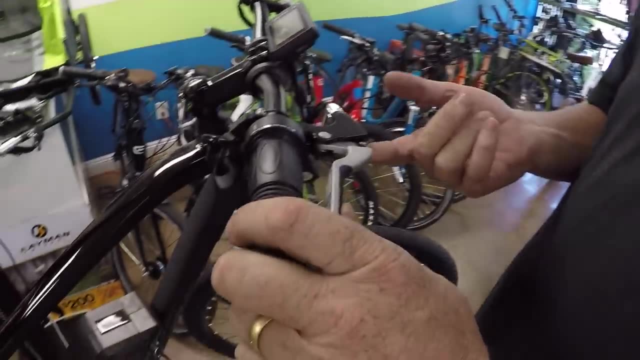 Yeah, another area would be cables. Like, if you get water into this area here, you probably want to shoot some lubricant back in there afterwards. Tri-flow works great, And some people actually just use grease in this area where your cables are. 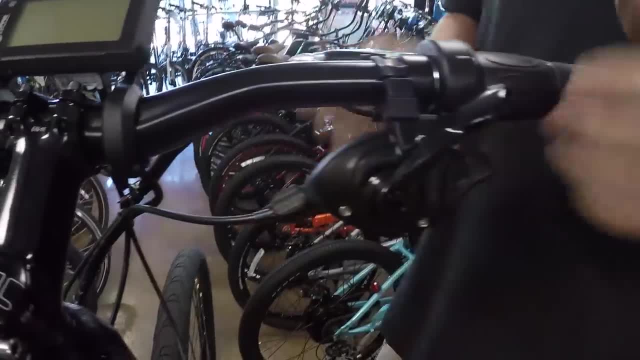 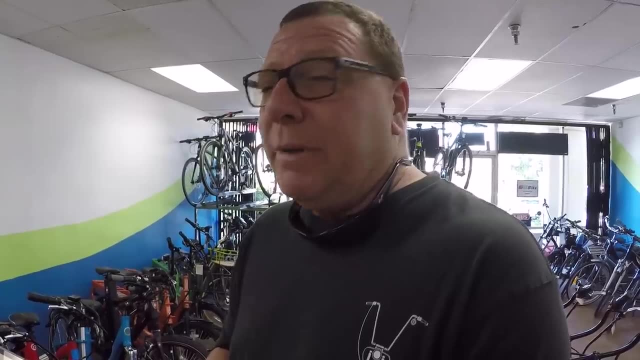 I'm really not concerned with anywhere that there's a cable, you want to try to keep it lubricated Over time. that can cause issues and your cable fray or actually fail on you. But just keep it lubed and you're good to go. 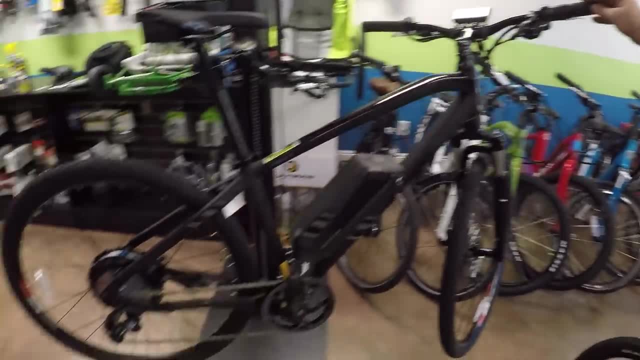 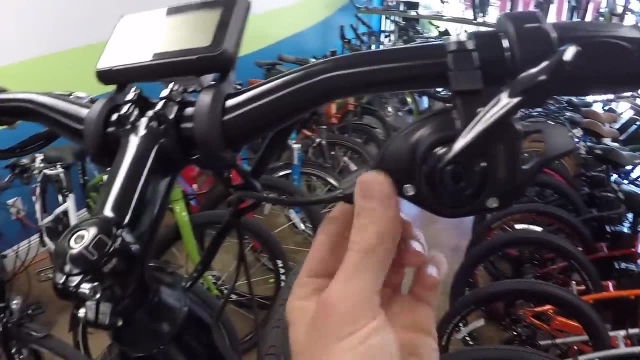 Okay, okay, sweet, Yeah. So we talked about a lot of different parts on this bike And I guess we touched on brakes earlier. but I wanted to reiterate that, in addition to this sort of finger adjuster for trigger shifters, a lot of times brakes have that. 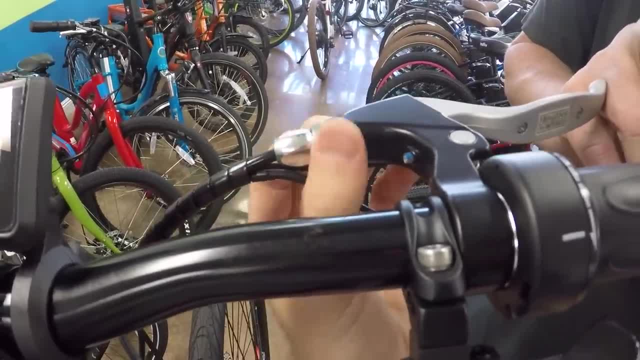 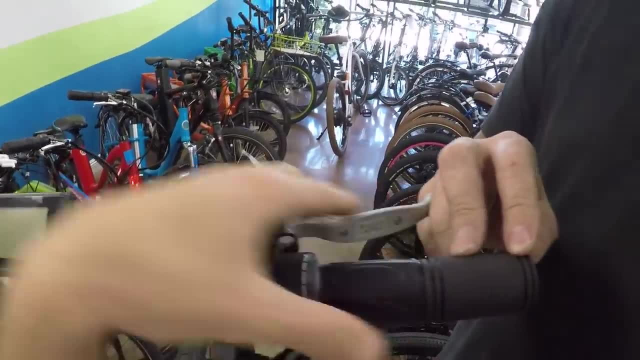 as well, And you can kind of unscrew the far point and then tighten the inner point And see what that does. is it like stretches the I don't know sleeve, And then it means the cable has to travel further. So over time, as the cables stretch and you're pulling the brake lever all the way back and 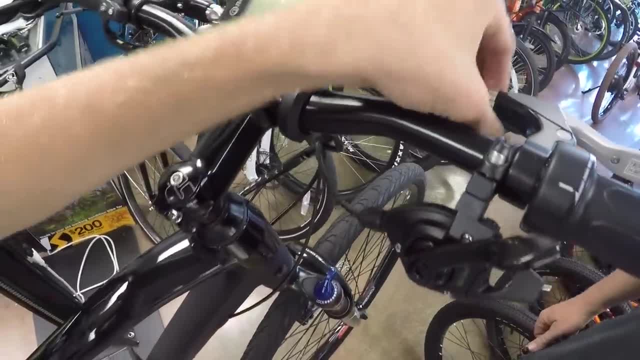 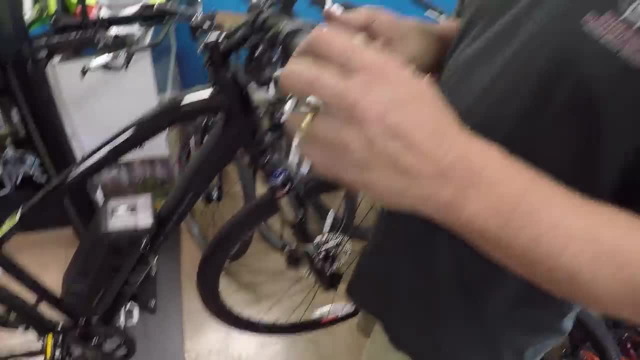 it starts to almost come in contact with the lever. well, that's when you can loosen this up. And you know what? As a shop, I leave that adjustment for the customer. I always make the adjustment down below And if you do need to make that quick adjustment, this is the simple area for the customer to 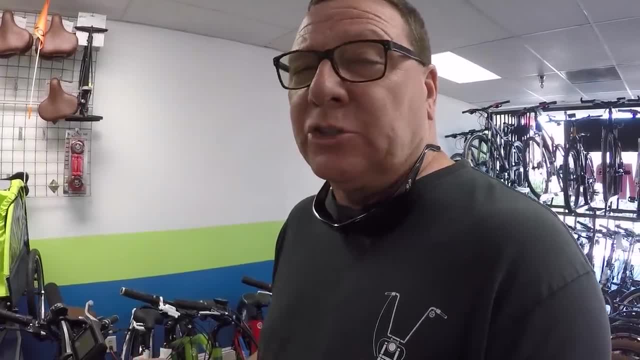 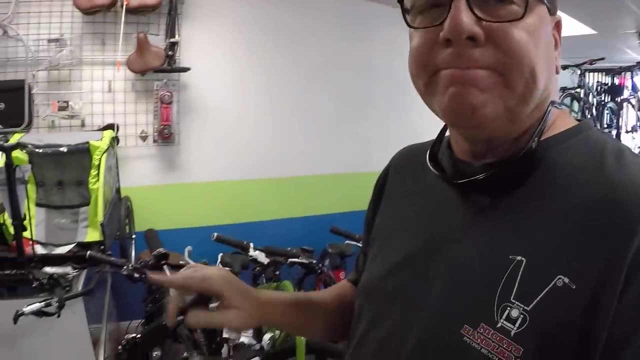 do, And that's like you said. it's just extending the length of the housing, which is shortening the length of the cable, which will bring the arm up down below and bring the caliper more in contact with the brake pad. Okay, 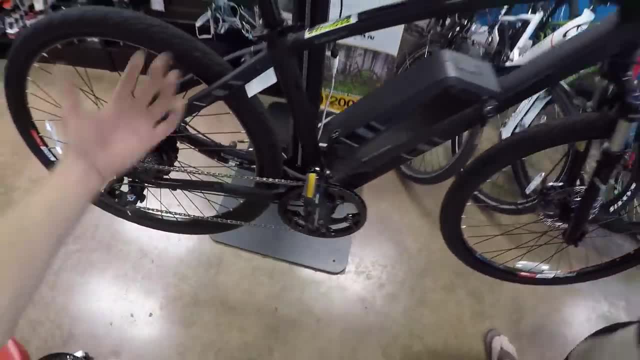 Any timing you know as far as, like every 50, 100 miles, get the chain kind of lubed up. You know it depends on the kind of riding you're doing, If you're going off road and you're mountain biking. 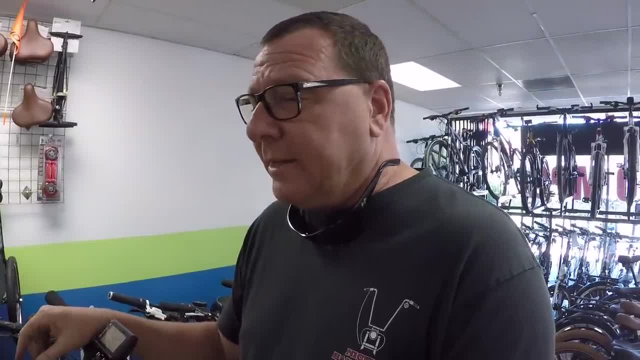 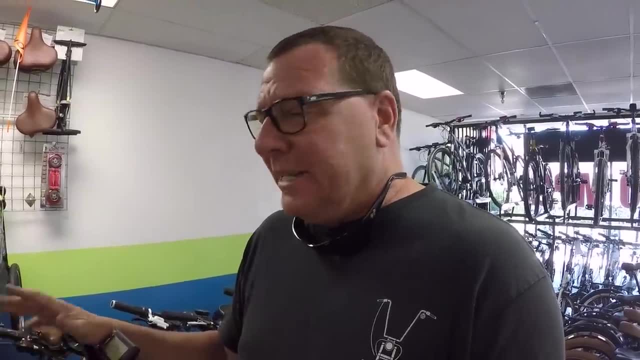 Every time That's a good time I recommend. But if you're riding on a road bike, I was commuting 40 miles a day and I could go a couple hundred miles before. I think 50 mile interval is way too soon. 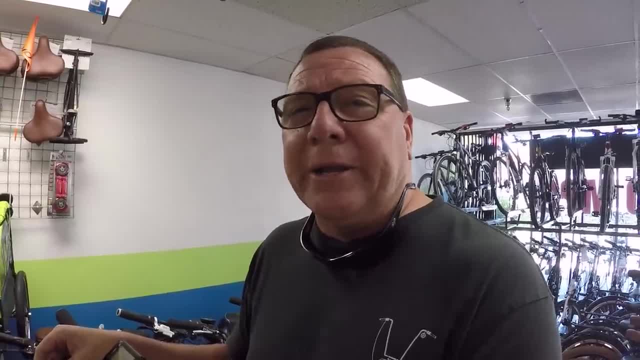 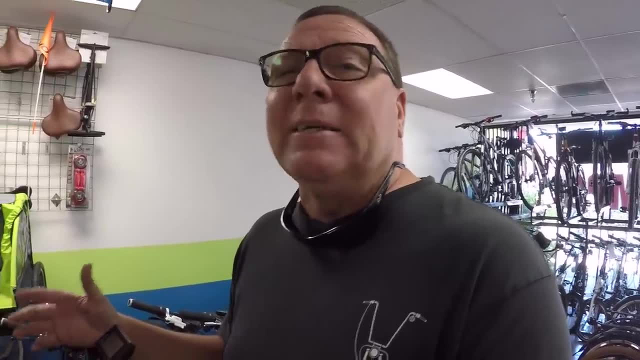 You can go a couple hundred miles before you have to really like check your bike and lube it. You know you don't have to be that diligent on it unless you're going off road and you're getting it really dirty. Every time we go camping, the bikes come home, they get washed, they get lubed and then 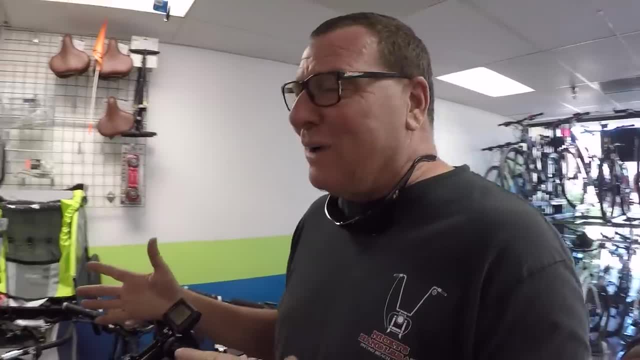 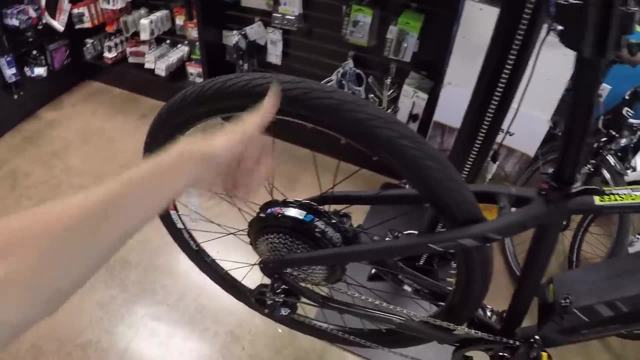 they get put back out here as demos on the floor because we like to ride our bikes and know you know the Specific sound. What's going on? Yeah, Have a good idea. So that's Oh. and when you're lubing it, I think don't you kind of switch through the gears a little? 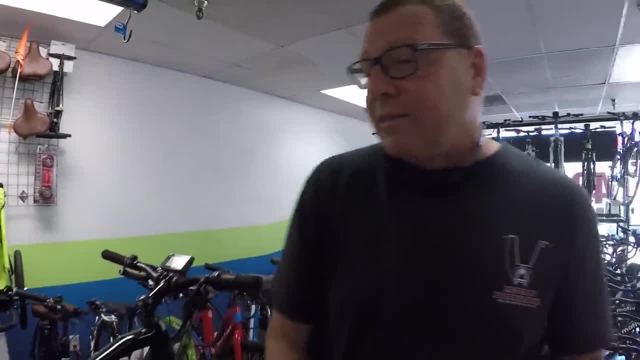 bit so that it gets Absolutely. I run them up and down. And let's talk about one last thing. I think that's really important. Probably one of the biggest, scariest part of owning an electric bike is: I'm out on the. 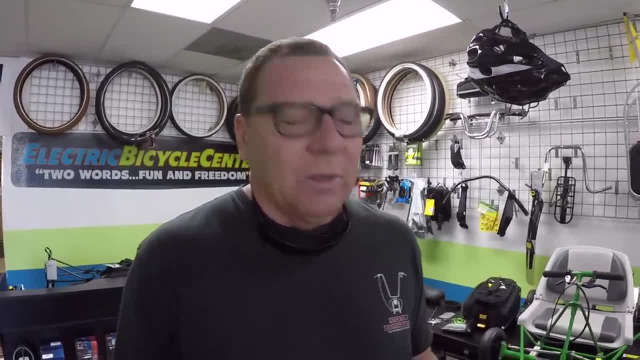 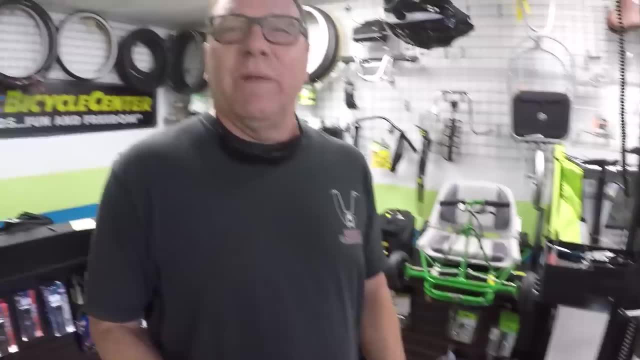 trail, I got a flat tire. Oh my God, What do I do? Yeah, I do not. recommend you try to remove the whole wheel and, and, and, and, you know, change out a tube. I recommend carrying a patch kit nine times out of 10.. 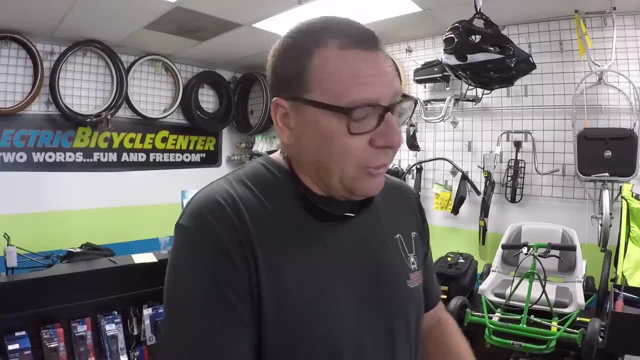 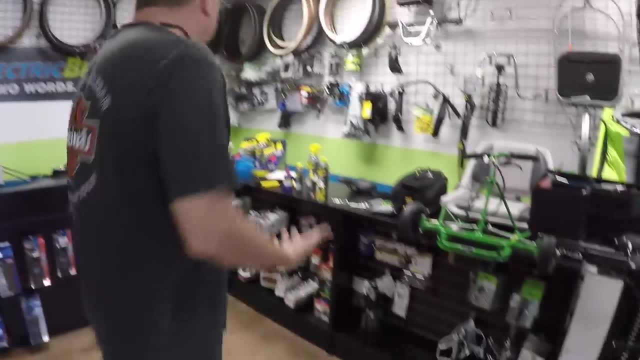 It's a puncher, It's not a blowout. Yeah, And you can change and fix the tube without removing the rear wheel. What I mean by that is: take a tip, just take a pair of really simple tire irons with you. 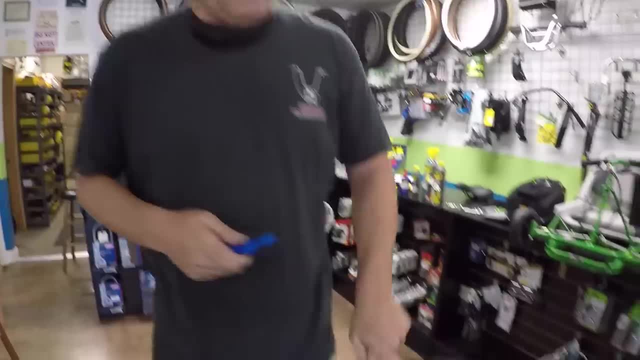 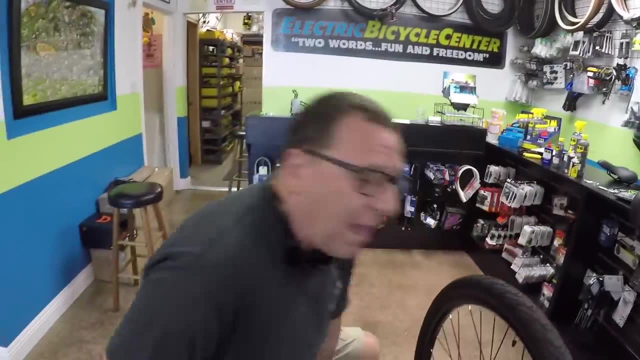 That'll remove the bead on the tire. Okay, And the bead bead is like that's the tight, firm edge right here, So tucks into the rim right. So you're going to pull that bead off on one side of the tire and you're going to try to. 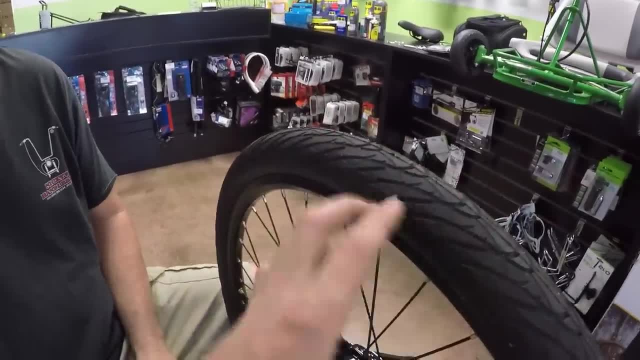 find where that puncture is. And I think, yeah, you kind of listen like if you can look and see, and if you got a little hand pump, you're pumping it up and you're looking for that hole is nine times out of 10 too. 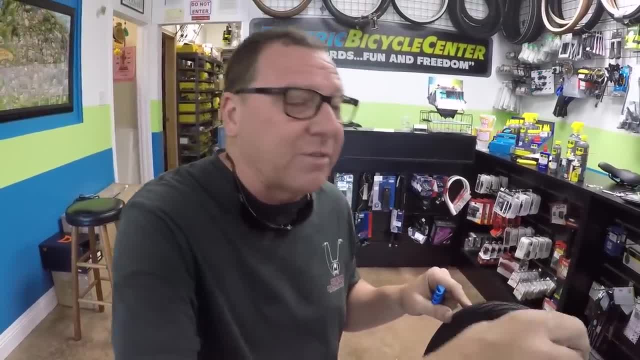 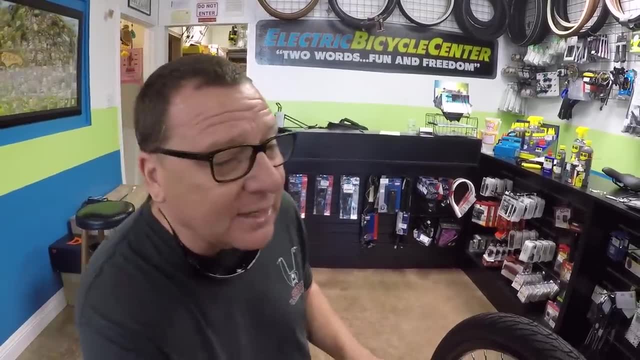 You'll find the puncture point because the thorn will still be in there, The staple will be in there, The piece of wire will be in there and you're like, obvious, Okay, That's where I want to look from this point, where the stem is, I'm looking for it. 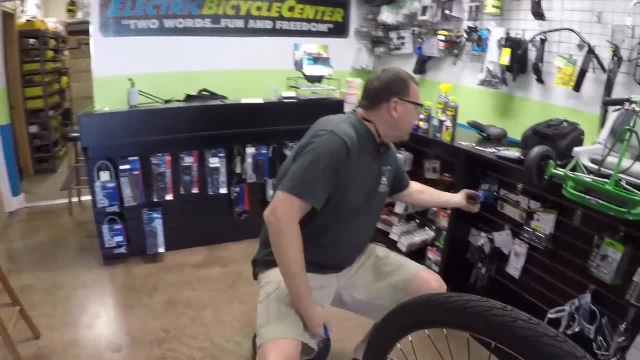 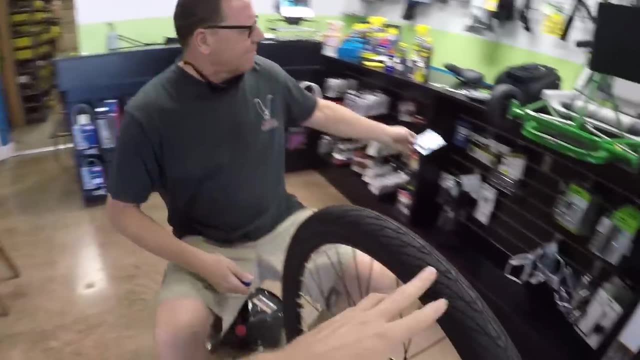 You pull the bead off, you find it. then you're going to patch it. Okay, I just want to throw in here This is my own personal brand of advice. Uh, sometimes if the thorn isn't there and you're kind of listening for it and you're- 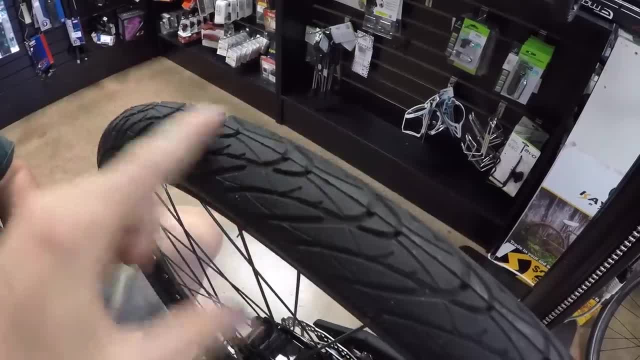 hearing, but you're not sure where it is, like kind of lick, you know, or spit on the, on the tire, And then you see it like bubbling right where it is. I'll put it up really close to my face and your face is more sensitive. 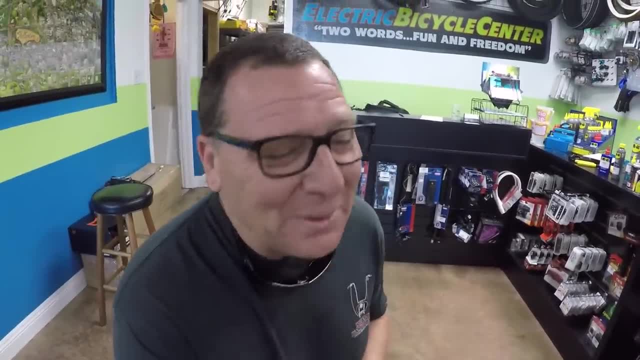 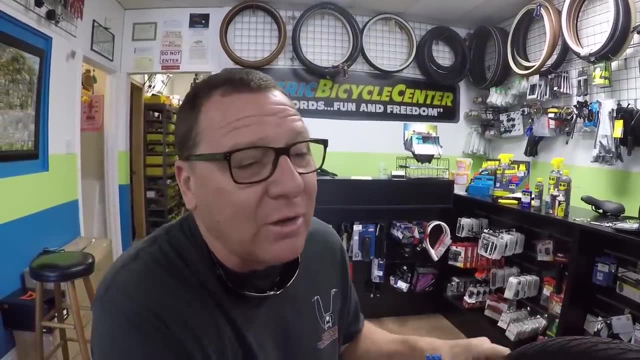 You're going to feel where that air is hitting you And then you've got to deflate it. put your patch on their weight, put the and nine times out of 10, you can put the bead back on without even using a tire. iron with a bicycle tire. 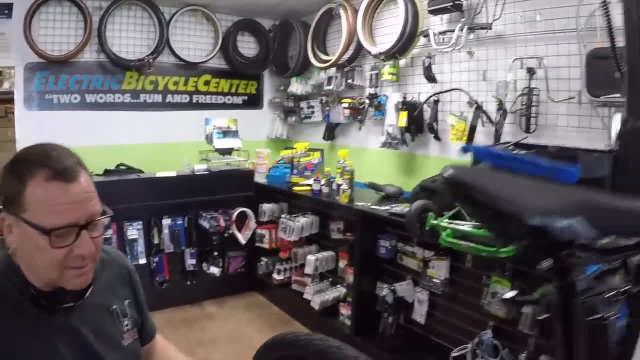 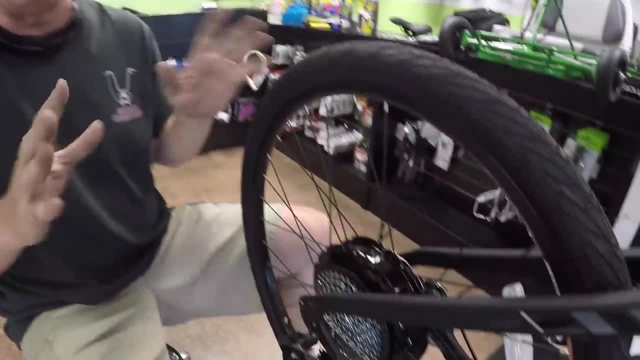 Okay, So that makes it easier And you don't have this daunting process of: oh my gosh, what do I do? How do I get my rear wheel off? I'm dealing with the wiring harness now to let the bike shop. let the bike shop take. 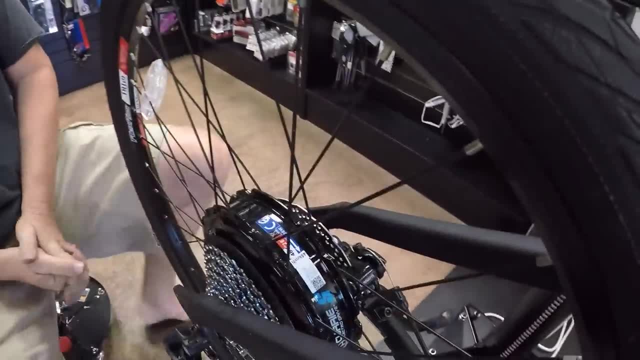 care of that for you. It's funny you say that too, Cause we were talking about the disc brake being lined up before. I've had it where- if everything was perfect, and then I took off like the front wheel and I put it back on. 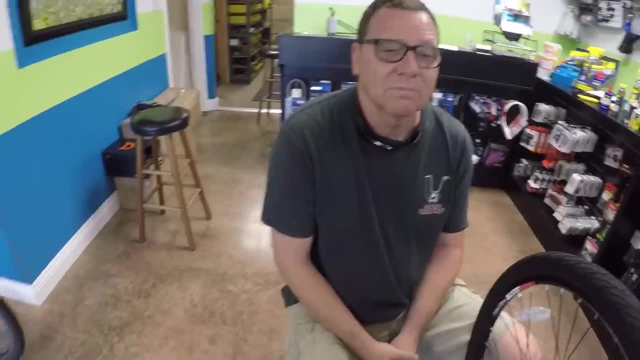 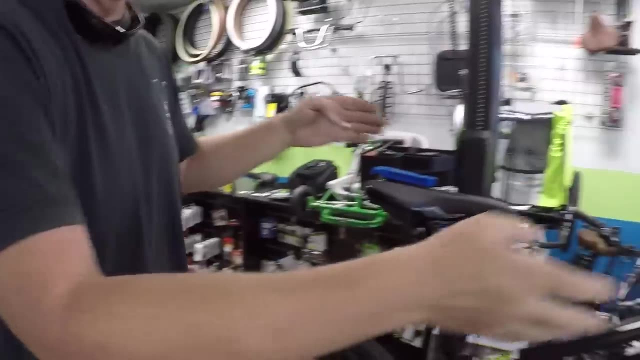 tightened it up and then the disc brake was rubbing and it's it's like trying to line those things up, especially on the trail, and get it spinning freely. It's a little more difficult, So you take the brake upside down, use your seat and your handlebars. 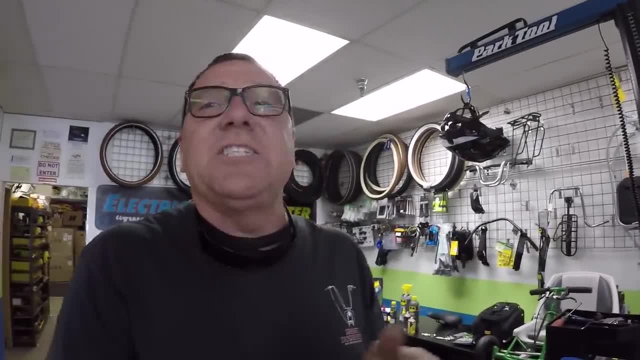 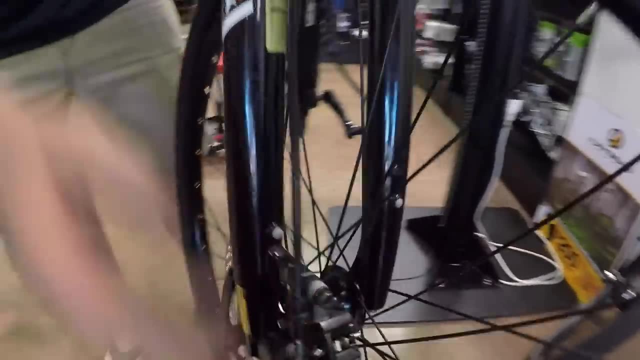 When you drop your wheel and make sure that it's all the way down on the dropout. If it's still rubbing. what you do, court, is this: check it out. There's two bolts right here and here on on every brake caliper. 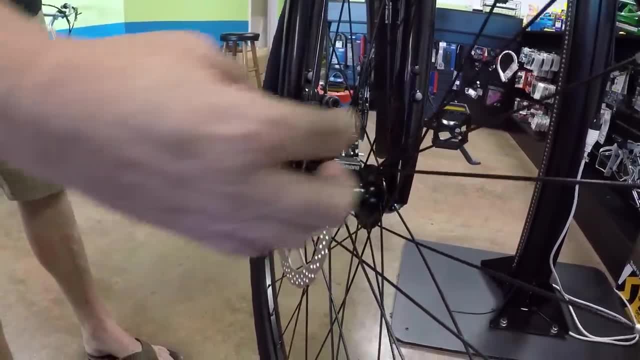 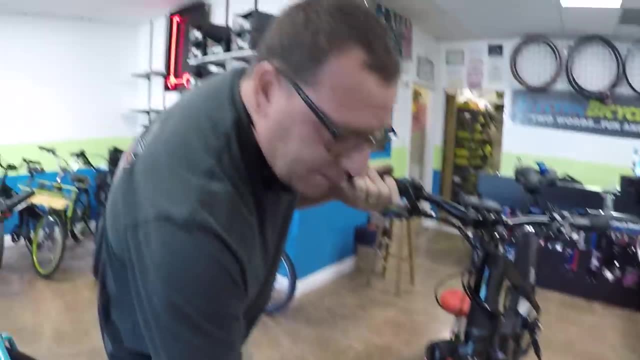 These two bolts, when you loosen them up, free, up the brake caliper where it floats around, Oh cool. Then you pull the brake lever And as you pull the brake lever, that's going to center it, Centers it. That's brilliant. 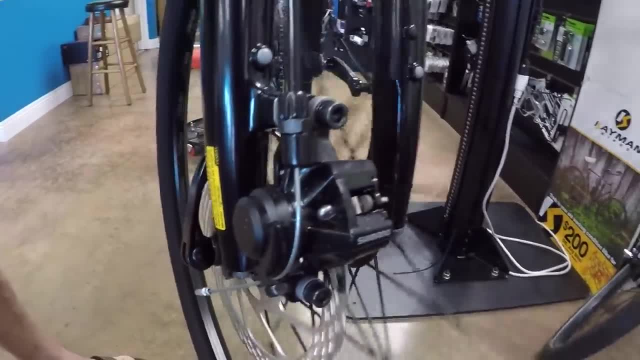 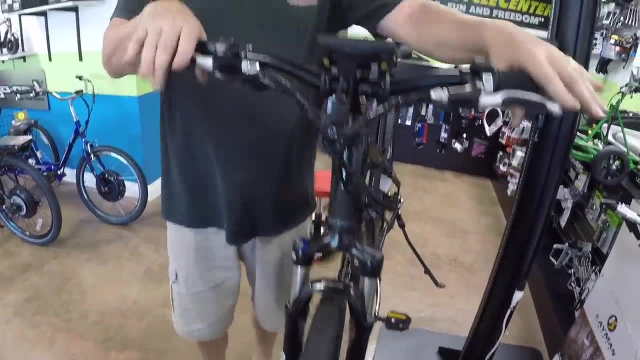 Then tighten the other two bolts down, release And again nine times out of 10, it'll be lined up and it'll spin freely for you. Perfect, Perfect, I love it, I love it. All right, A couple of little tips here at Myron's: 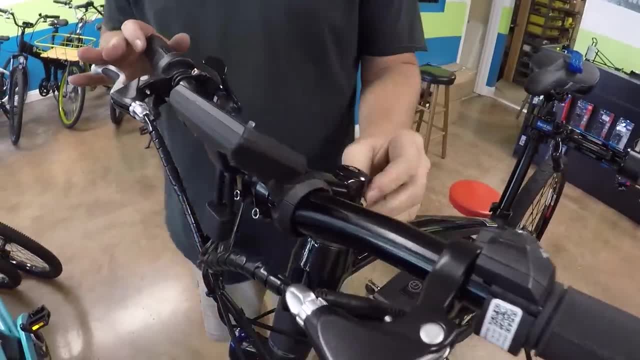 Also headstay. Sometimes your headset will get a little bit loose. Make sure it's tightened down and clamped down here, because other- yeah, I've seen it before- where, like you, could, you know, squeeze the tire between your legs and pull on the. 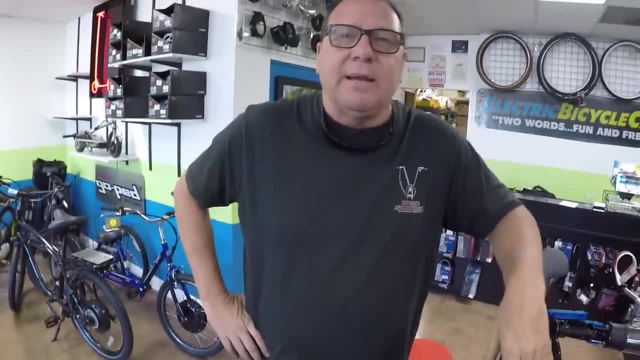 handle and twist it. If that's not, it's not tight enough, then it needs to be tightened up. What are some tools that that maybe you carry here? You can point out that you recommend always taking with you. you want a helmet, right? 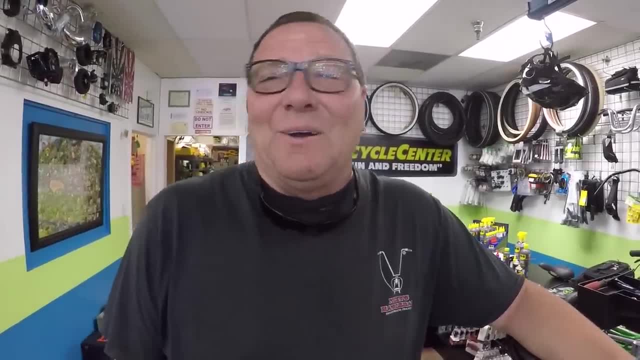 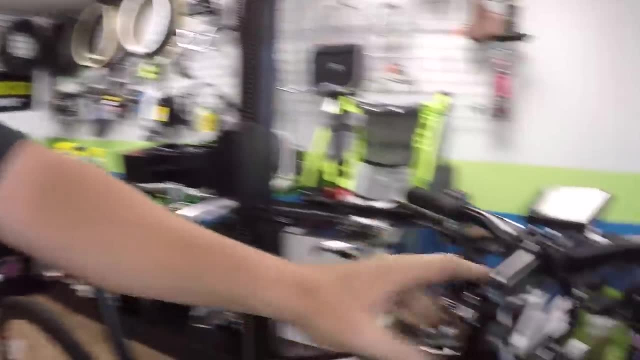 That's not a helmet, That's not a tool, but Well, in a way I guess it is. you know it's protecting your most important, valuable asset up there, Your brain. Sure Allen, wrench, set tire, irons, patch kit. yeah, a little. all you need is two. 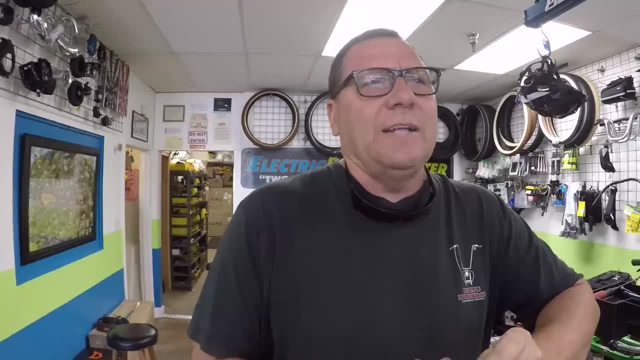 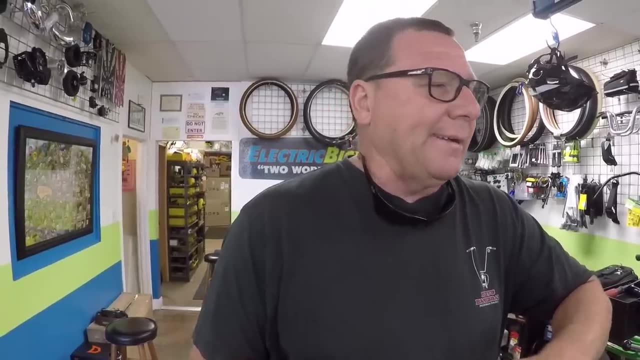 Tire irons, Allen wrenches- And what size Allen wrenches should I take? Three, four, five and six? pretty much dove everything on on most modern bikes. You might want to take a 10 and an eight, but rarely do you even need to use that. 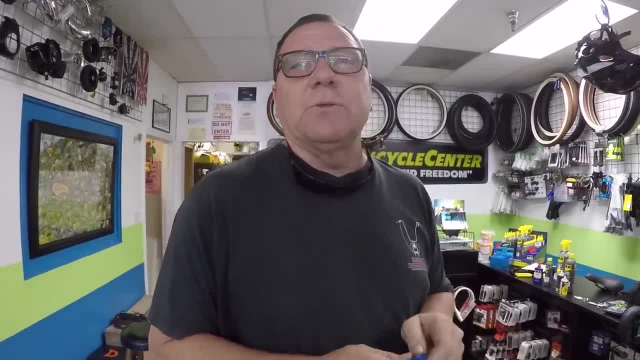 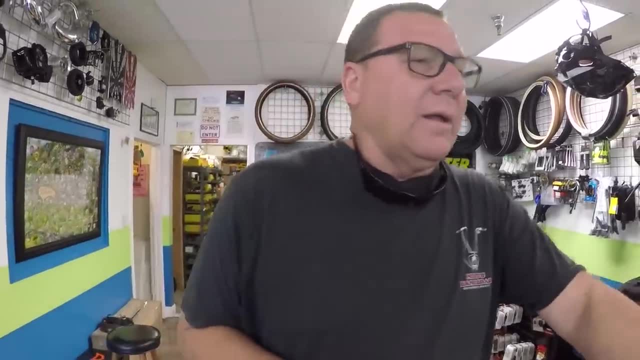 You use those, those tools? I personally carry those type of tools with me every time I go on a bike ride and I haven't been stranded yet. The mini pump thing: Do you feel like you take a pump, or Absolutely A mini pump or a CO2.? 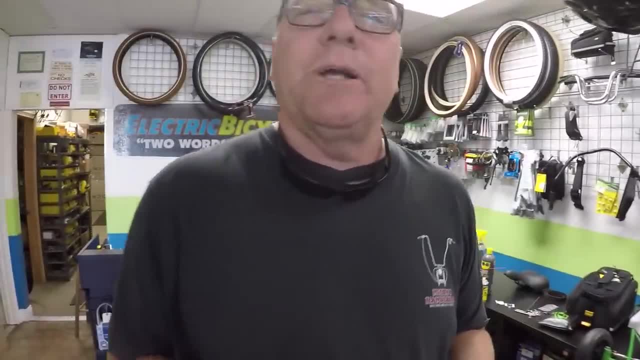 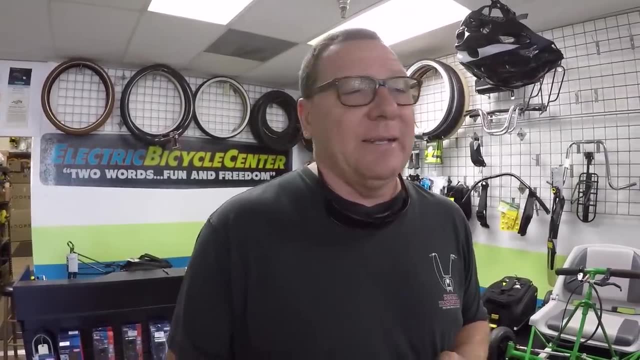 I prefer a mini pump myself. That way I can adjust tire pressure on the trail And I think one of the most important tools you can carry around with you is a cell phone. Not a bad idea to remember to have one of those. That's the emergency backup last resort. 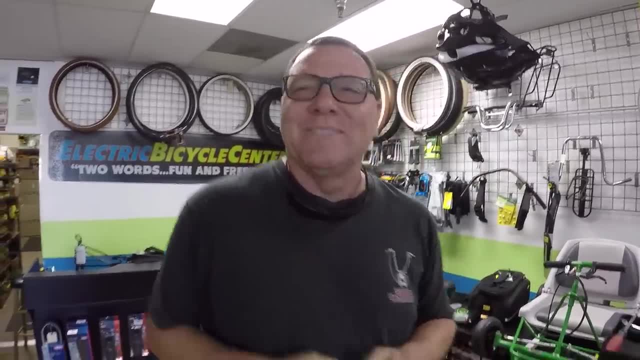 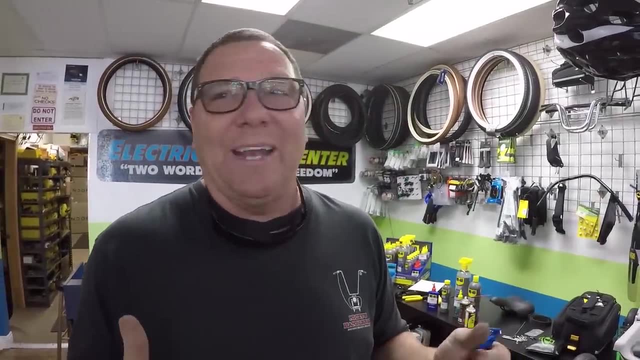 Pull out the cell phone and call your buddy up and say: come pick me up. You can text NASA with pictures and be like: what do I do? I'm stranded And the mission control. I've actually had people call me on and I'm working and I literally will go out and pick. 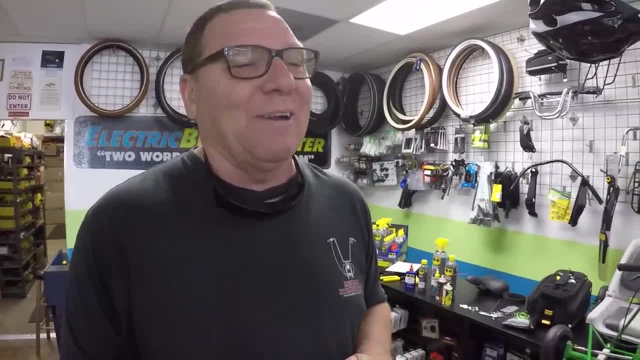 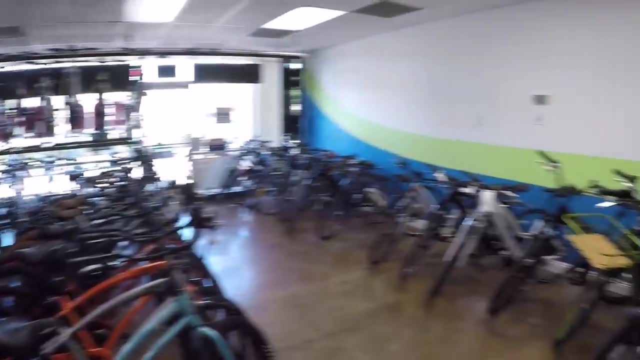 them up if they're within the vicinity of my store and get them taken care of. And I should say again, thank you so much for Sam. lets me review all the bikes and stuff that he has here. He's got one of the biggest shops that I've seen. 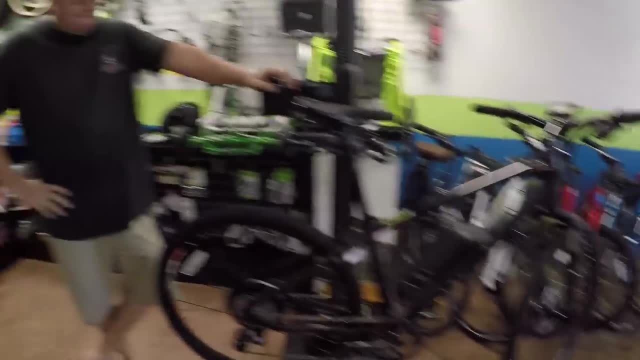 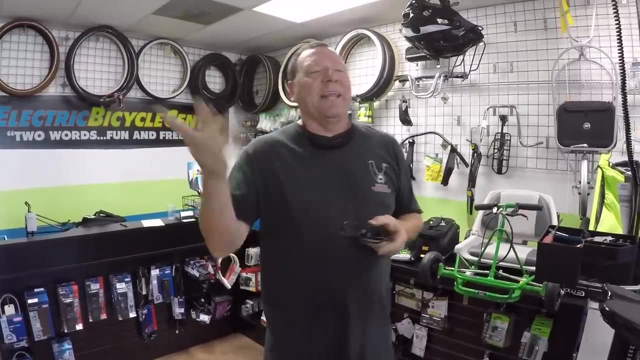 He always gets new stuff, very experimental that way, And you try it out And you go camping, you go to the desert. here We're in Fullerton, California, So it's near LA. We're kind of near LA, Yeah. 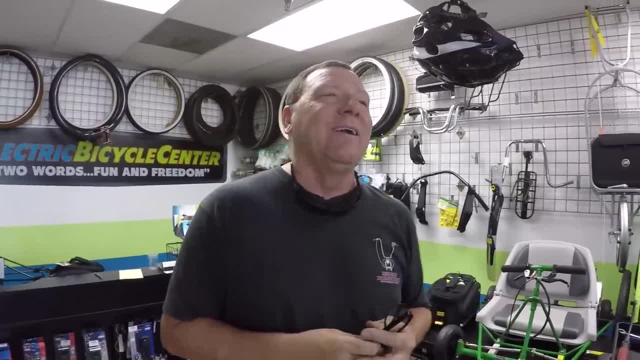 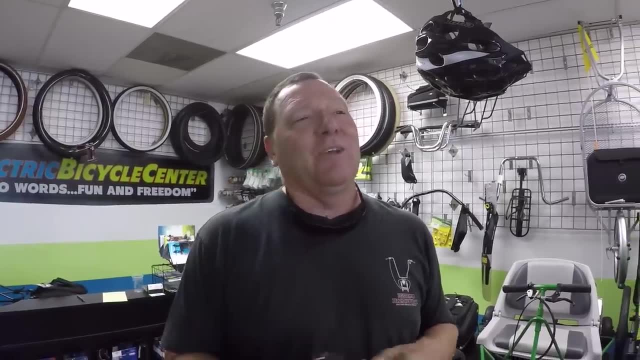 We were camping out at Canyon RV park about 20 miles away and we stayed two weeks there. That's a 40 mile commute And every single day we come into work and grab a different bike and go back out. And so we got a lot of bikes with a lot of impressions from a 250 watt, 24 volt folding. 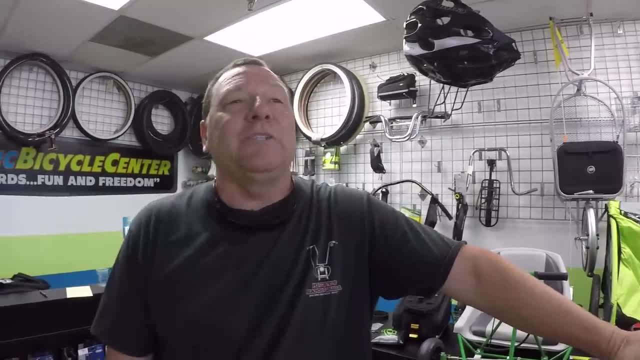 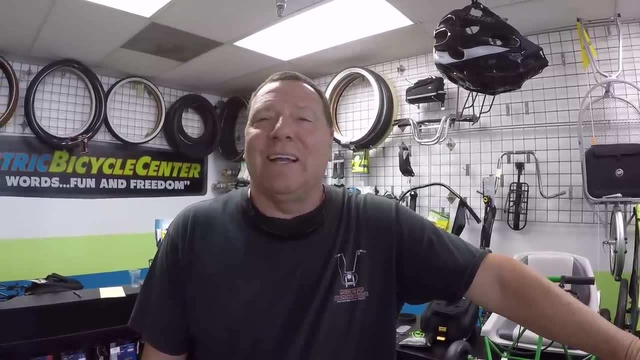 bike to bikes that hit 30 miles an hour And it was interesting on the Santa Ana river trail with the various people and the various looks that I got and the various comments, But mostly positive, And you're a big guy, I mean you know your significant other, Kanika, she's. she's a little bit shorter. 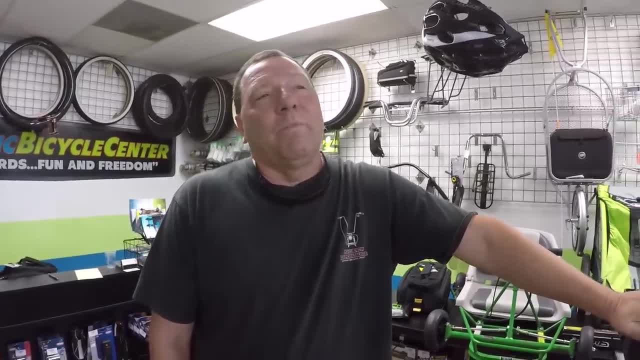 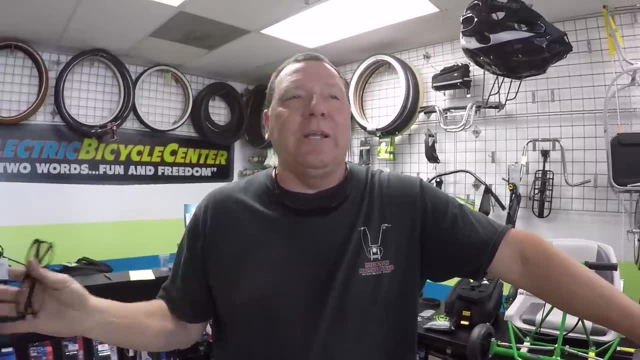 She's a little bit lighter And so you're getting kind of the his and her perspective. We're at opposite ends of the spectrum, So at a hundred pounds and 260 pounds that gives you a good, you know, range of body. 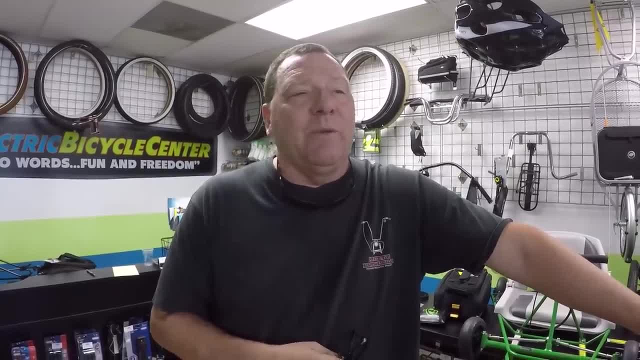 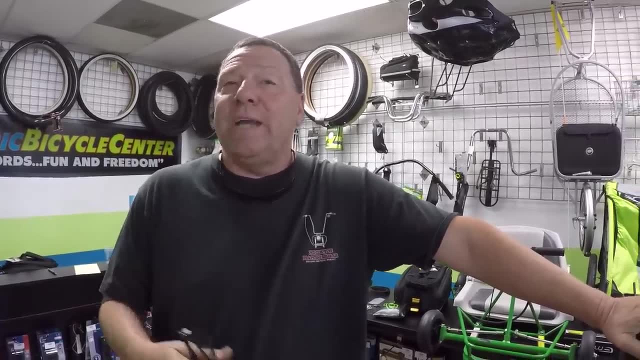 styles and sizes, as to how the bike's going to perform, And we would try different levels of pedal assist And in some cases, Yeah, We would go there and back and not even pedal the bike just to see what kind of range the battery had. 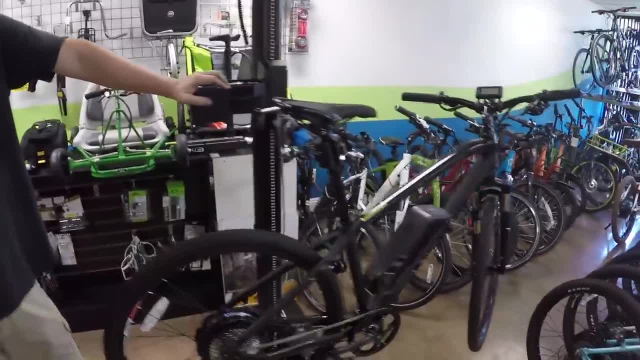 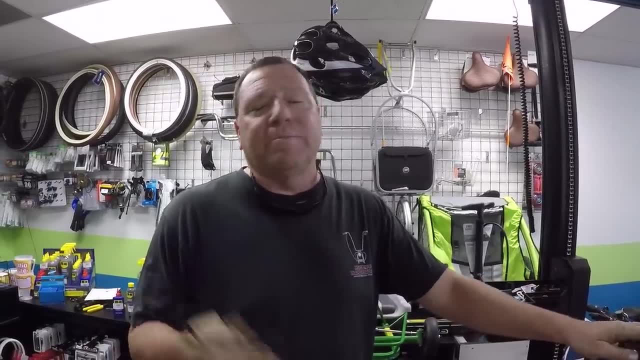 Yeah, Well, well fun. Any any last thoughts on maintenance and all that. If you don't, if you have a question and you're not sure, call your local bike shop, call your local electric bike shop And most people are going to have the answer to your question. 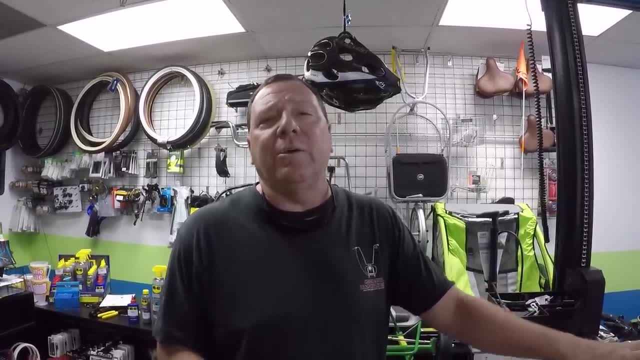 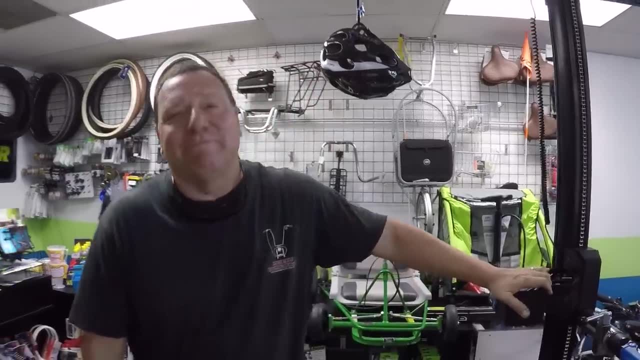 Don't be afraid to give us a call. We're more than happy to inform you, educate you and get you down the road. So the smile comes on and you're having fun like a kid again riding your electric bike. Thanks, Sam. 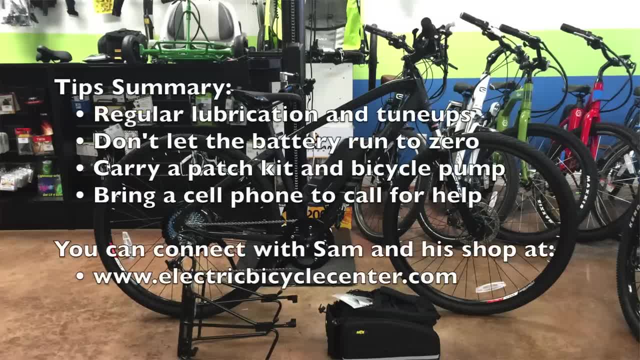 Bye, Bye, Bye, Bye, Bye, Bye.